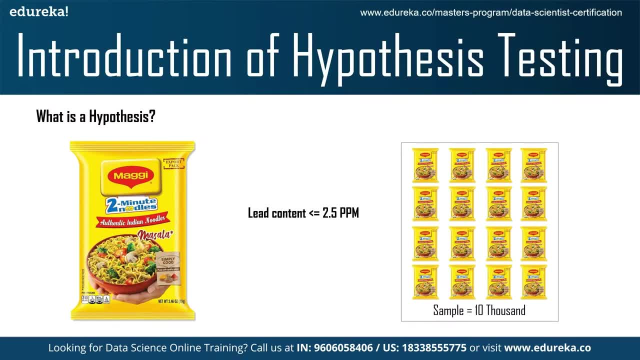 of Maggi noodles and that's how they found out that there is excess lead in Maggi noodles. So this is how it becomes a claim: By extracting a sample through a very big population, because the government regulatory body cannot do tests on all the packets of Maggi noodles, so they 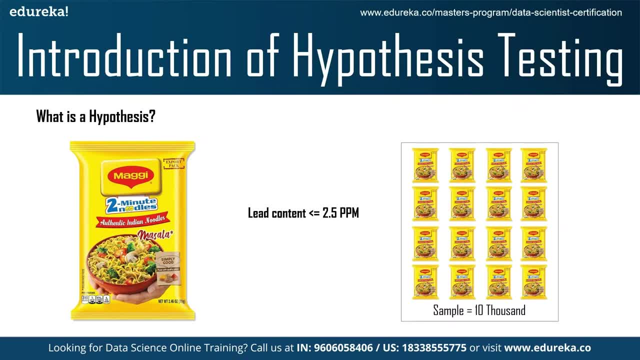 extracted out a small sample out of a very big population and they made a test out of it, And that's how they reached to a conclusion. That's how they claimed that Maggi noodles contained excess lead. So the process of extracting our sample from a big population and conducting a test on it is called hypothesis. I hope. 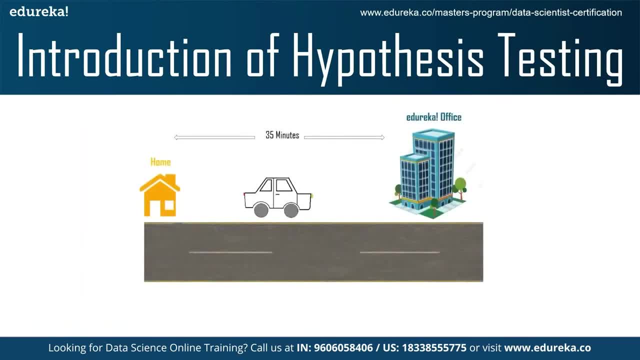 it's clear. now We can also look at another example, Like a survey being conducted on Edo-Reca employees. The average commute time of an Edo-Reca employee to reach office from home and then going back to the office comes out to be 35 minutes on average. But it's 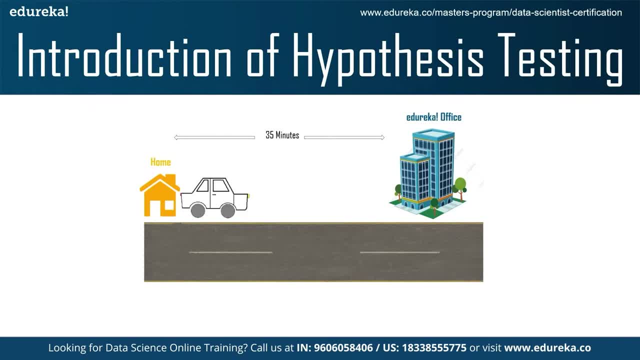 an average Means there are employees which are taking time as 10 minutes also, some are taking time as 50 minutes also, 1 hour also. Some are taking just 30 minutes, 40 minutes And then some are taking 30 minutes. For example, some are taking 30 minutes, 40 minutes, 30 minutes. 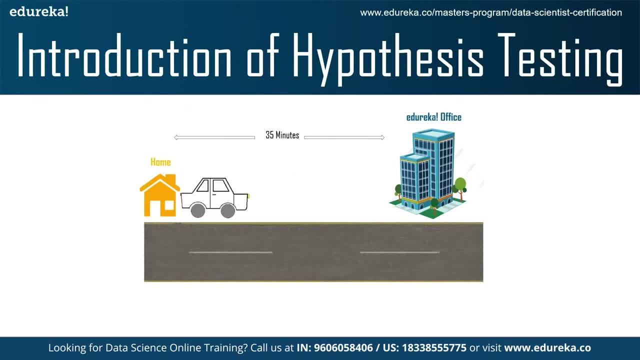 30 minutes, 40 minutes also. so we found out that we conducted a survey on 100 employees and we found out the average compute time to be 35 minutes. so this becomes a claim. this is the status quo. so this is how the hypothesis has been formulated. now let's understand what is hypothesis testing. 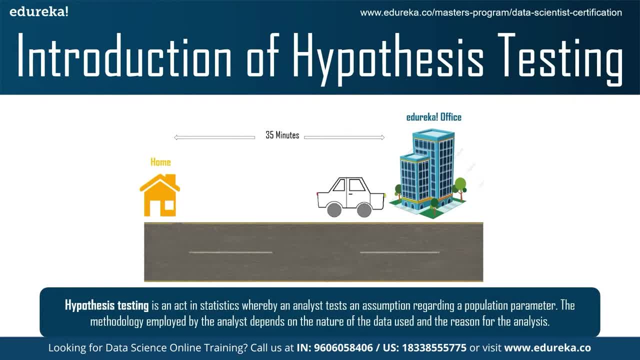 so if you conduct a test on this hypothesis, that's what hypothesis testing is. so hypothesis testing- if i frame it, it becomes hypothesis testing- is like used to confirm your conclusion about the population. through hypothesis testing, you can determine whether there is enough evidence to conclude if the hypothesis about the population parameter is true or not. now let's understand. 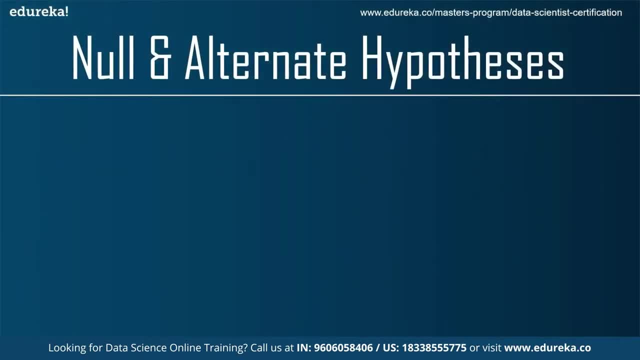 the null and alternate hypothesis. so we will understand this with an example of criminal trial. so suppose there is an accused which has done some crime and now judge has to decide whether he has done the crime or he has not done the crime. so they are like now, two hypotheses, you can see. 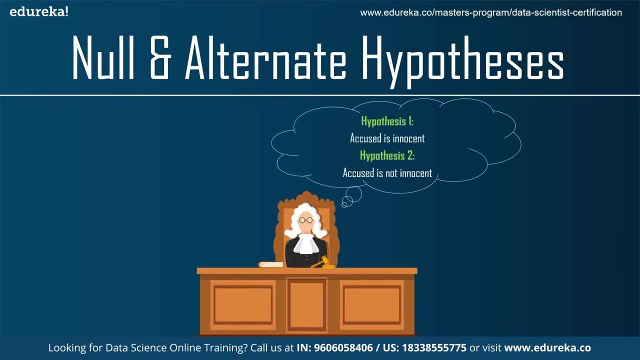 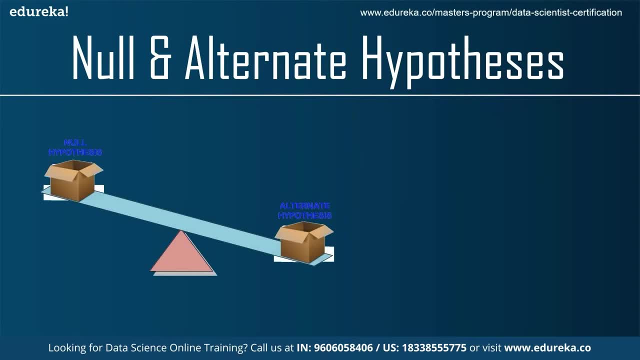 the first hypothesis is that accused is innocent, he hasn't done the crime, and the second is that the accused has done the crime and he is guilty. so you can see here like there are two opposite hypotheses here. so the first one is null hypothesis, denoted as h naught. 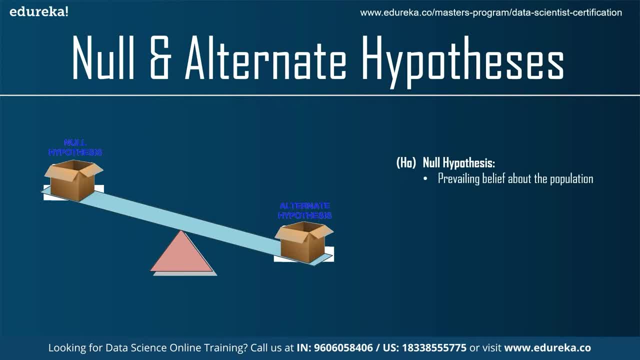 which is a prevailing belief about the population. it states that there is no change or there is no difference in the status quo, means there is no difference in the situation according to which the accused is innocent and he is just a member of society and he hasn't done anything wrong. now 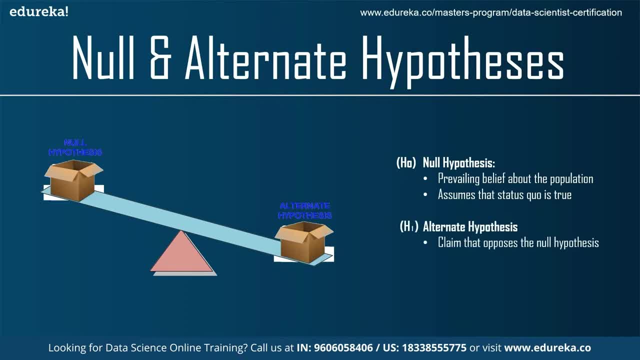 second one is alternate hypothesis, denoted as h1, which is a claim that opposes the null hypothesis, which means the accused is innocent, which brings a change in the situation, a difference in the situation. now, if you look at the null hypothesis, you can see that the accused has done the crime and the 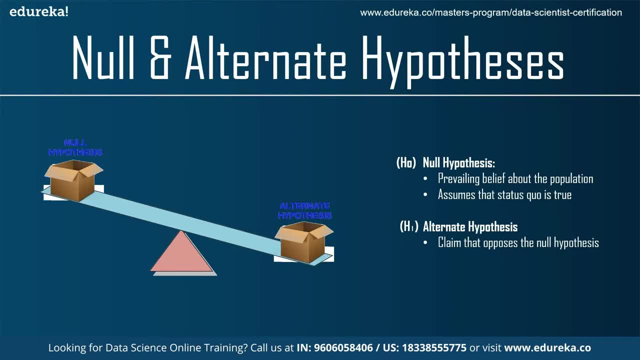 opposition says that he is innocent, so that is the assumption that he is the accused, and the position that he has been given by the police is like that fall, if you remember the older example which i gave you of mega noodles. now the status quo here is, if you remember, the null hypothesis: 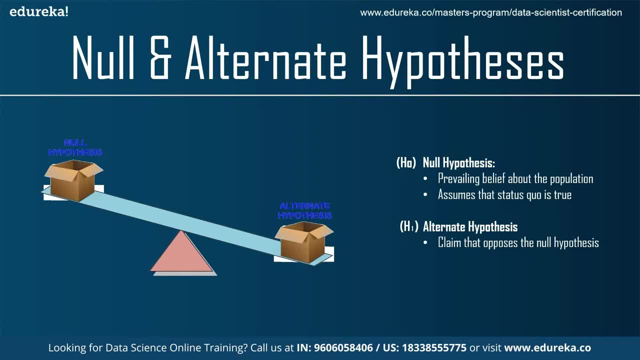 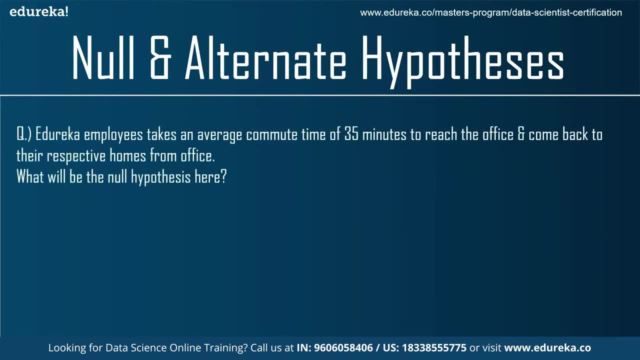 here is that the lead in the food product, means in the mega noodles, does not exceed the maximum limit, that is, it does not exceed the 2.5 ppm. and the alternate hypothesis will be: lead in the mega noodles does exceed the 2.5 ppm limit. that is the maximum limit. now, if you remember the example of 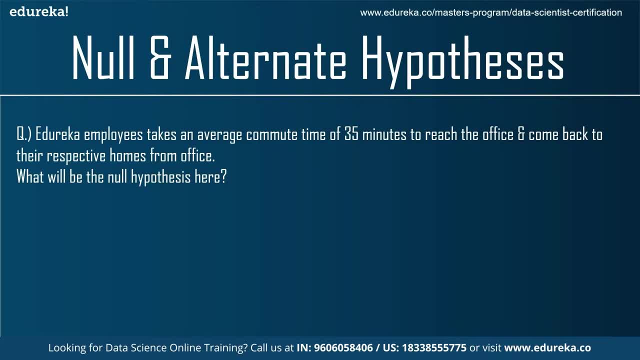 commute time, which is taken by them as 35 minutes. but suppose now the claim is: after some research or survey we found out that it's taking more than 35 minutes. so now can you please tell me which one is? the null hypothesis will be in the situation like? i will give you the option. so the first. 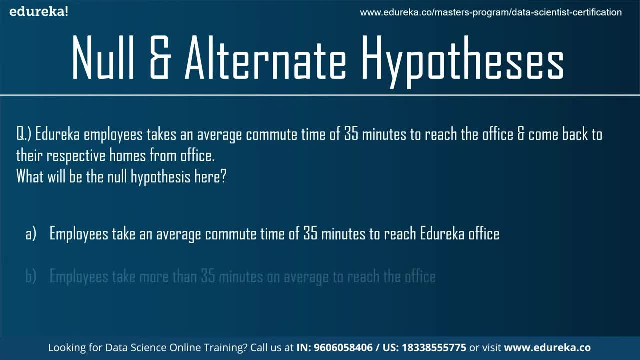 option is like employees take an average commute time of 35 minutes and option b is: why is take more than 35 minutes? so you can pause this video right now and you can answer the question in the comment section below. now you see the outcome of the communal trial example is like the null. 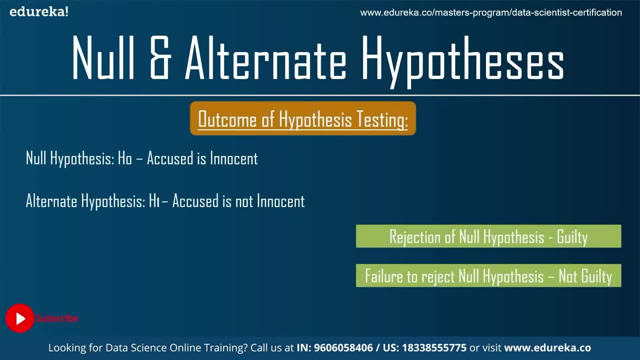 hypothesis: accused is innocent and alternate hypothesis: the accuser is not innocent. so if you see here the rejection of null hypothesis will be like guilty, because that is status quo, there is no change. but if you reject the status quo, which means the accused is guilty and the second 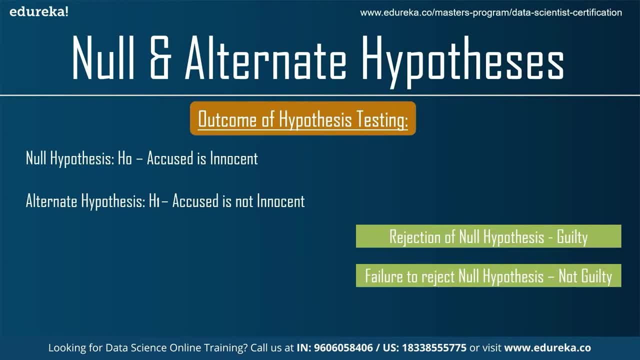 is failure to reject the null hypothesis, which means the accused is not guilty, which means like we don't have that enough evidence to reject the null hypothesis. but remember this thing: that in any way there cannot be a situation where you accept the null hypothesis and the failing hypothesis. 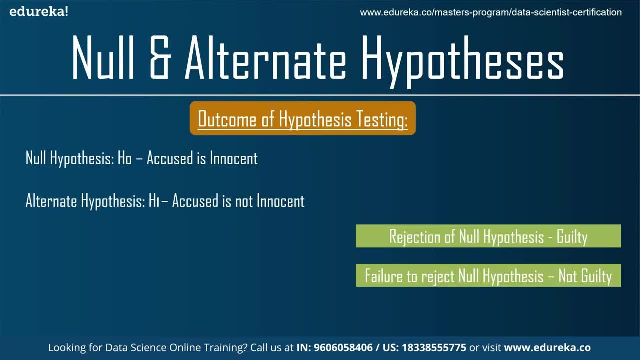 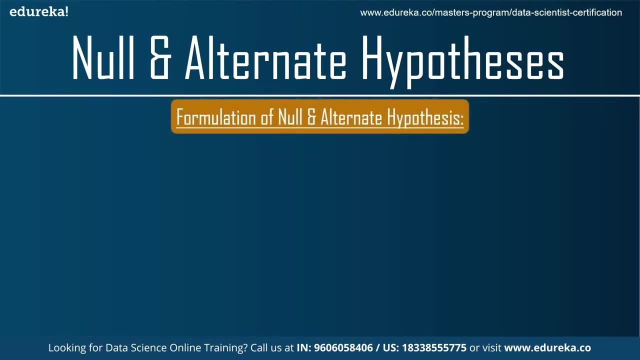 either the null hypothesis. the only situation is, you don't have enough evidence to reject the null hypothesis. now we have to understand this important concept, that is, formulation of null and alternate hypothesis. so now we will understand how to formulate null and alternate hypothesis. so if your claim statement has words like, at least at most, less than or greater than you cannot formulate, 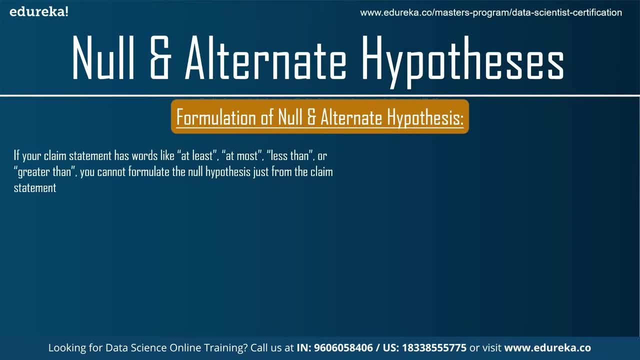 the null hypothesis just from the claim statement, because it's not necessary. the claim is about the status quo means always about the status quo. so you can use the following rule to formulate the null and alternate hypothesis. so the null hypothesis always has the following signs like: equal to, or smaller than equals to, or greater than equals to, and the alternate hypothesis always has: 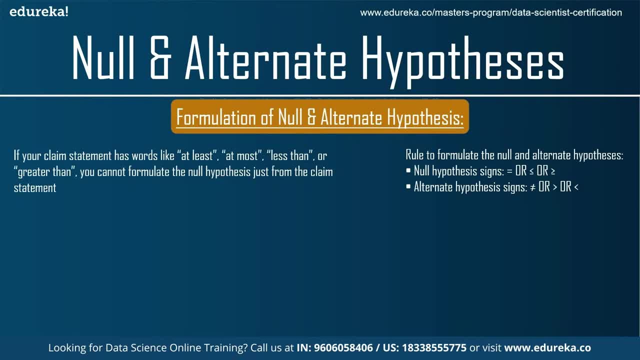 the following signs like: not equal to or greater than or lesser than. keep that in mind. this is a very important thing. now let's see an example of flipkart. suppose the plant claimed that its total valuation in december 2020 was at least 20 billion dollar. here the claim contained: 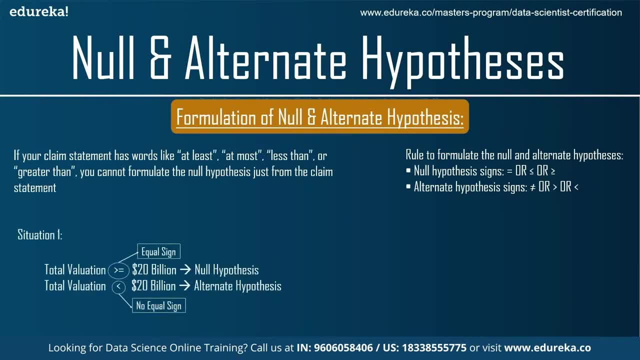 greater than equals to sign. so the null hypothesis is the original claim. the hypothesis in this case can be formulated as, like you can see here, total valuation greater than equals to 20 billion dollar, which is null hypothesis, and total valuation is smaller than is 20 billion dollar. you can: 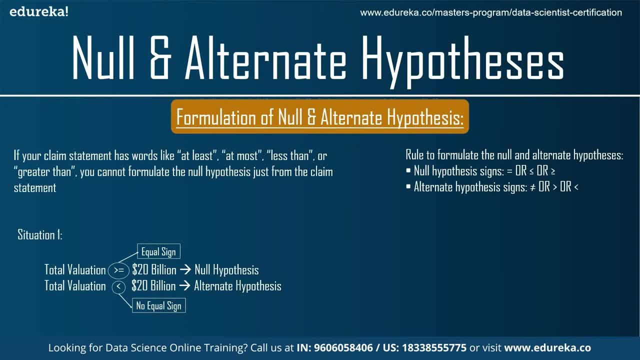 understand the difference between the signs. i have told you the signs which are used in null hypothesis and alternate hypothesis. you can see: the equal sign is there and there is no equal sign in the alternate hypothesis. similarly, in situation two, you can, like flipkart, claim that the total 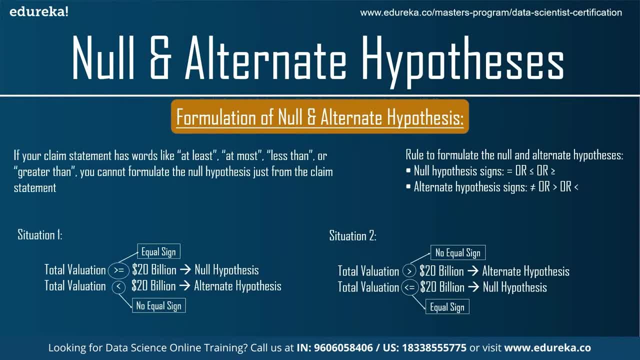 valuation in december 2020 was greater than 20 billion dollar. here the claim contains greater sign, so the null hypothesis is the complement of the original claim. so the hypothesis in this case can be formulated, as you can see, like: total valuation: greater than 20 billion dollar, which is alternate hypothesis. 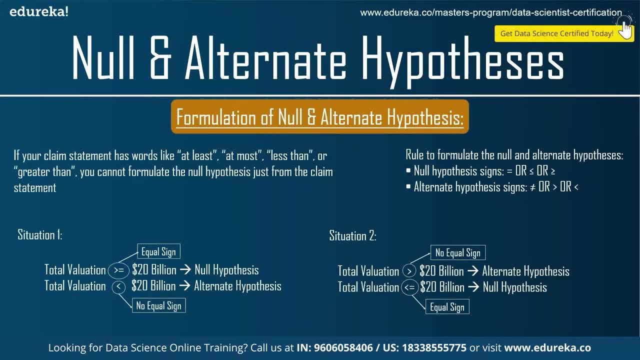 and total valuation which is smaller than equals to 20 billion dollar is null hypothesis. you can see the difference between the signs. to summarize this: you cannot decide the status quo or formulate the null hypothesis from the claim statement. you need to take care of the signs. in writing. the null hypothesis it always has to be. 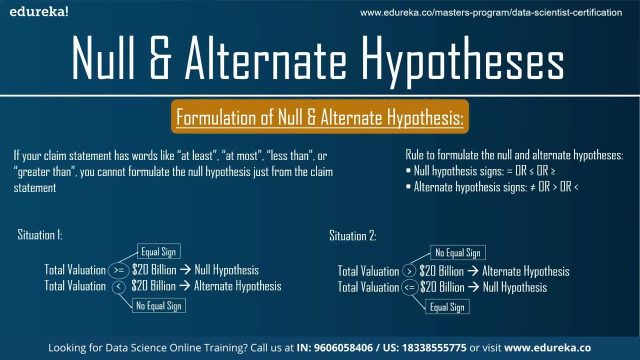 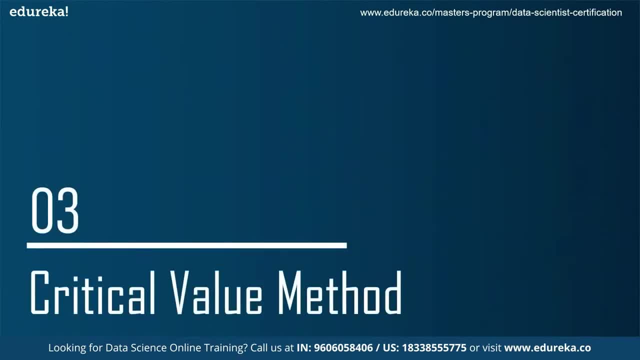 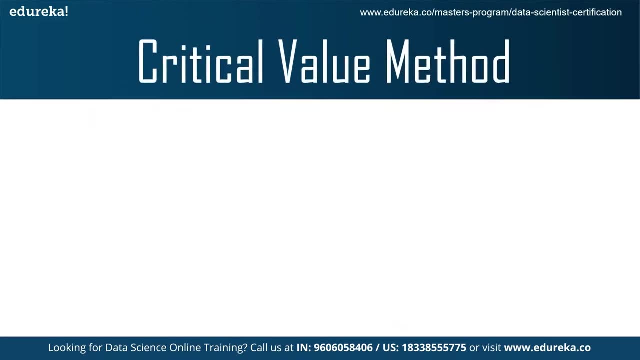 formulated using not equals to, or greater or smaller signs. once we have formulated the null and alternate hypothesis, the next most important step of hypothesis testing is making the decision to either reject or fail to reject the hypothesis. we will understand this with the critical value method, so we take here the example of archery. now suppose there's a friend of yours named avril. 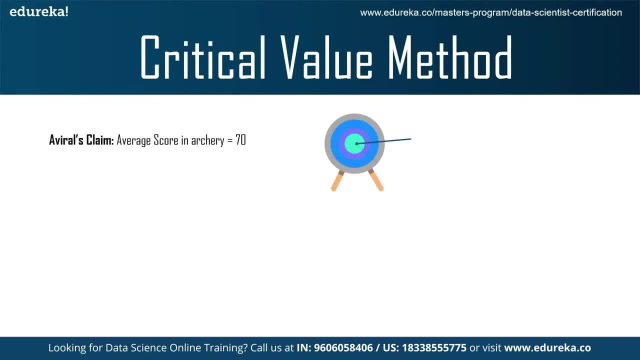 who likes to brag about his skills of archery. and he told like he has scored 17 archery. but you doubt his claim because you have a perception that he likes to brag about. you have this perception of avril that he usually brags, so you doubt his claim. so you can see like 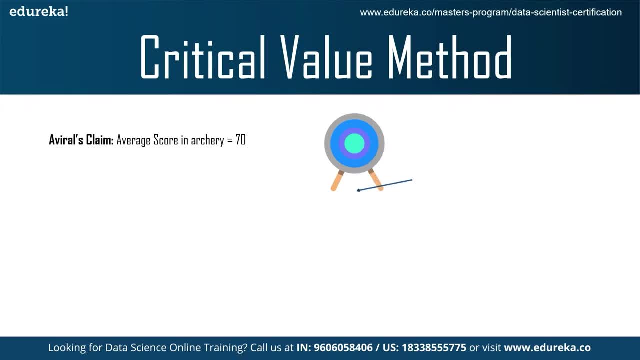 avril's scheme here is that he scored 70. that is the status quo means, that is the null hypothesis. so for clearing your doubts, just for the confirmation purpose, you played a match with avril, so you played like over five games of archery with him and you find that the average 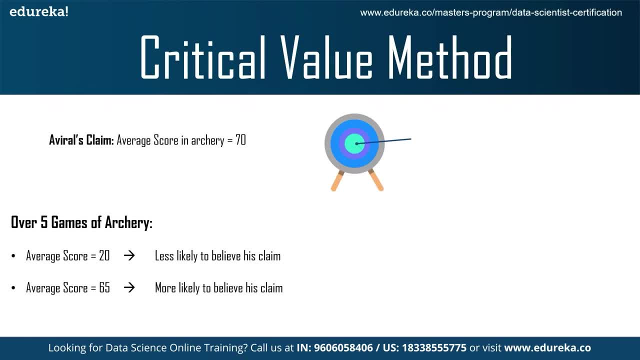 score of game is a 20. so which is like less likely to believe actual claim of avril if he gets 20 as the average score, because 70 is like far away from 20.. so you can like reject the null hypothesis, but the average score of five games is like 65. in that case you more likely believe his claim because 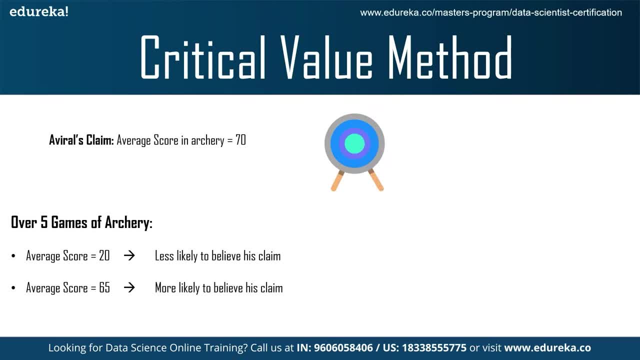 that is near to 70, or if it is more than like, even 70. like suppose he got 80 or 90, in which case avril is like underestimating himself. so we can see this graph here, so you can say, like the status quo is 70.. suppose, like the score we can say for the five games, he got a little lower, like we can. 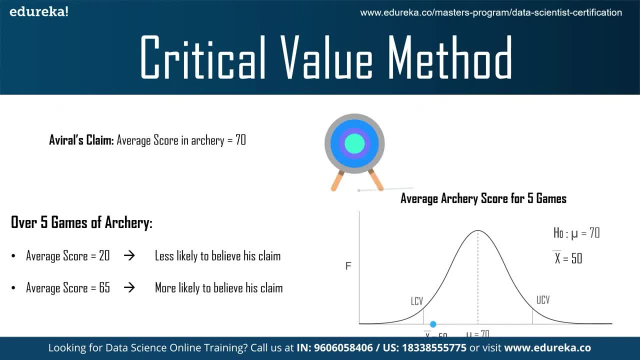 say around 55, 60, or say 50, we got. we can say like he scored 50.. now we have to understand like that: it is like a critical point where you will reject the avril's claim, or there is a critical point above which you will like accept the avril's claim. so we say these points as lower critical value. or 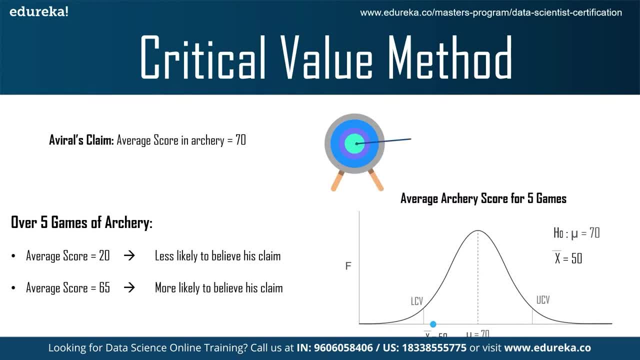 upper critical value, like suppose, if it is 50 or it is 55 or it is until 45, we can say just for example purpose- i am saying not for definitive purpose- if the score is 45 or 50 around. so we say like we can actually believe avril. but and if it is lower than that we can say like he was just 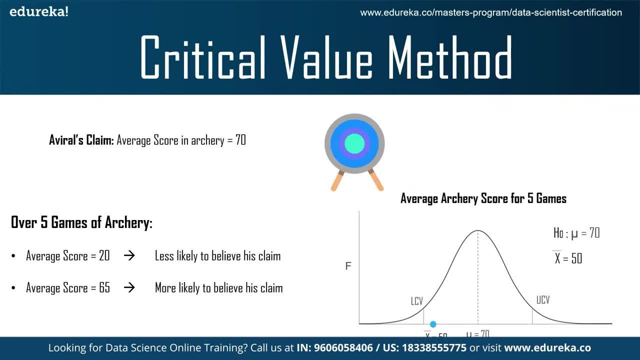 value around like 80 or 90, which is more than 70.. so if that is the value, then we'll also like accept the avril's claim. we can also say that he might be underestimating himself. so can you see this graph? first one in this: uh see, like if whatever the score comes out and red score is come under lower, 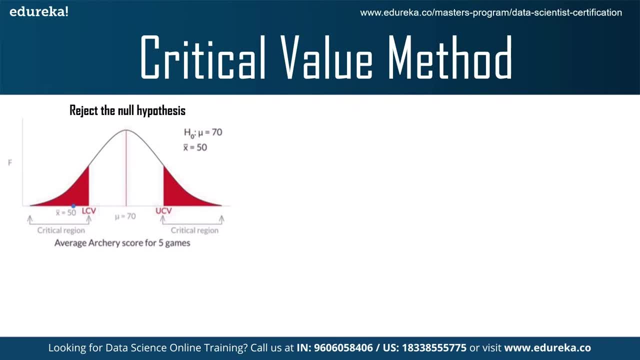 critical value. suppose you believe, like if he gets only 60 below, then that you feel like he is just bragging. so he got 50, which comes under lower critical value. so we say that avril actually, like was just bragging, and suppose you can say that avril is just bragging. and suppose you can say like: 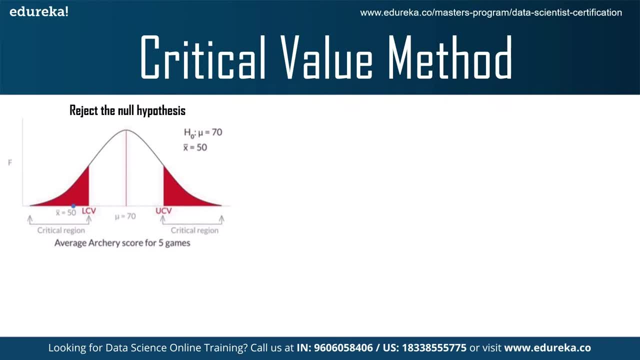 he got around 80 score, so you can say, okay, you are believing in him. but if you say like, suppose he got score of around 90 or 100, which comes into upper critical value, so you feel like he is just underestimating himself. so in that case, if the research hypothesis means alternate hypothesis, 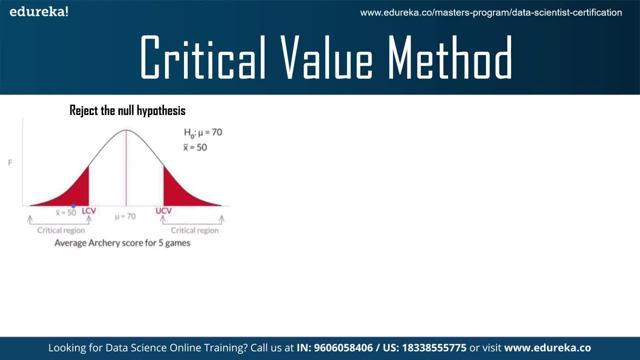 value comes under lower critical value, upper critical value, you reject the null hypothesis. and in the similar manner, if these values doesn't come under lower critical value or upper critical value, we say it comes under acceptance region, as you can see here, like 50 comes under acceptance region, so we accept the avril's claim. so in such a situation, 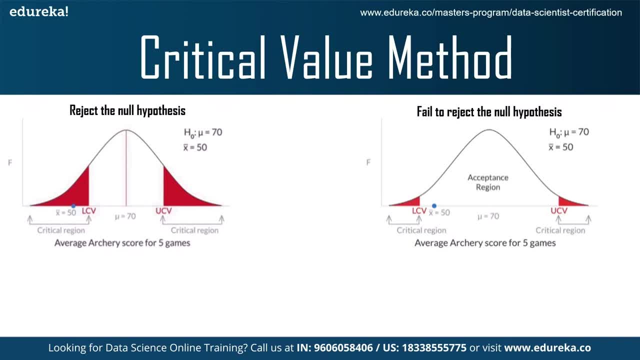 we fail to reject the null hypothesis. so these kind of tests where we have, like, both lower critical value and upper critical value, these kind of tests- we say it as two-tailed tests- which are mostly used in healthcare system, like suppose there's a medicine in which the paracetamol drug is required. 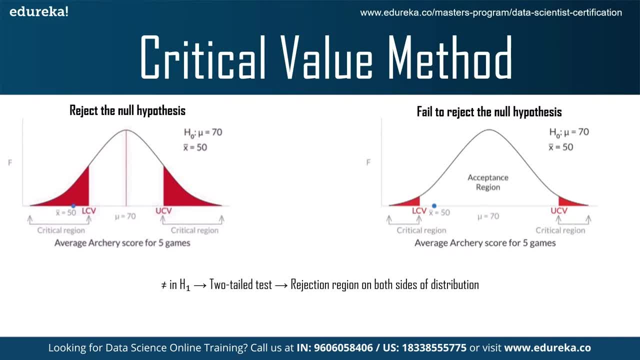 but there's certain amount of quantities required, like paracetamol which is used for curing pain and fever of a patient, and we require like 500 m for curing it. but suppose drug present in the medicine is just 300 grams, it will like decrease the efficacy of the medicine. 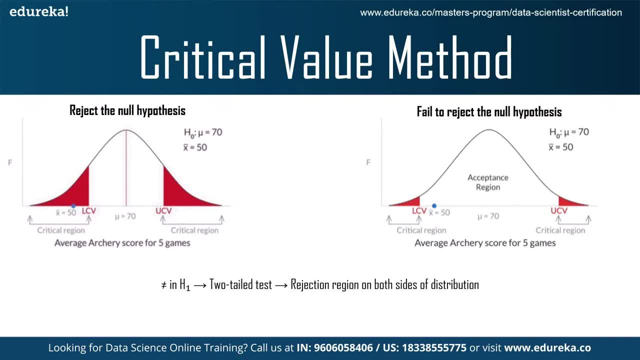 and it might not be useful for the patient. and like suppose there is a increase in the value of the drug, like suppose there is 700 gram or 200 gram, that can like do side effects to the patient. maybe it can like cause diarrhea or maybe cause other problems. so which is? 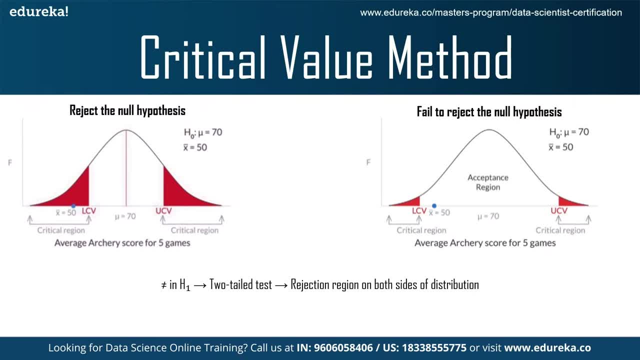 not a good thing. there is both lower critical value and upper critical value for that, so there should only be 500 grams of paracetamol, not more than that, not less than that. so that's the critical point. Now the second one is lower tailed test. so lower tailed test and like upper tailed test, both are there. 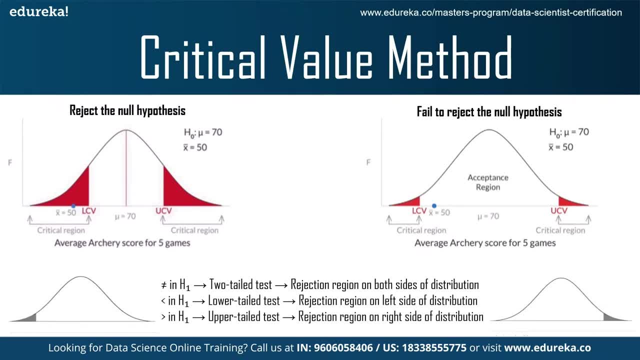 you can see how their graphs are shown. so these kind of tests are usually used in manufacturing companies, like we have taken example of Maggi noodles, where the government regulatory authority found out that the lead content in Maggi noodles has exceeded 2.5 ppm. so there is one kind of test. 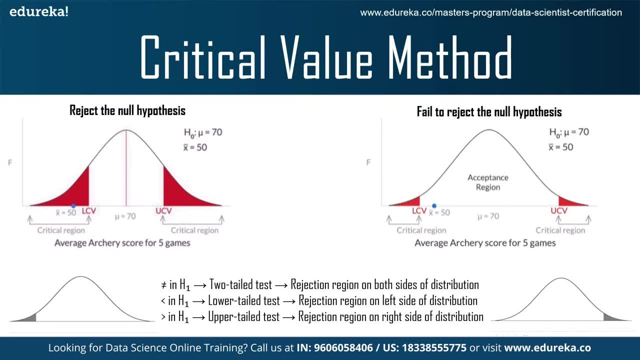 like in this. you can see like there was a upper critical value, like if it exceeds 2.5 ppm, that comes under upper critical value. there are like three kinds of tests in this one, As I have explained to you, like true tailed test, lower tailed test and upper tailed test. 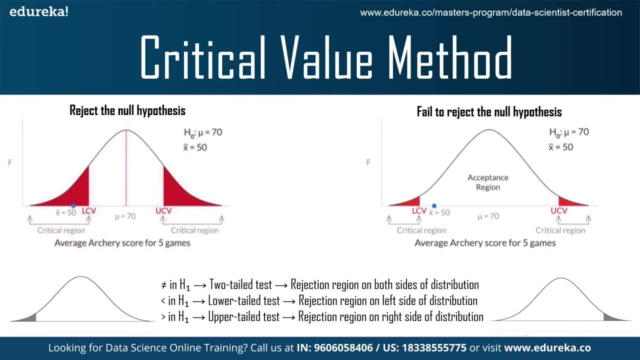 So you can see, like in lower tailed test, the rejection region is on the left side, as you can see on the left side of the graph. and if you see the right side of the graph you can see the rejection region is on the right side of the distribution. that is for upper 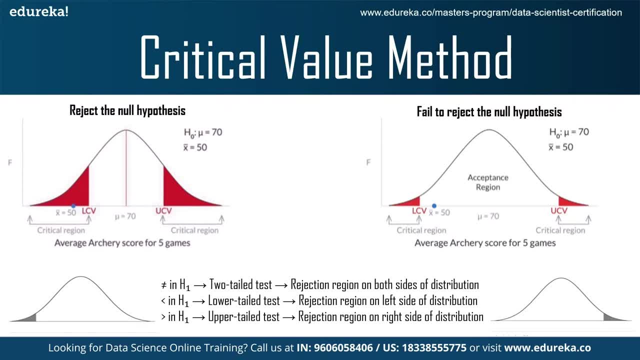 tailed. Now that you have an idea of acceptance regions, critical values- lower critical value, upper critical value- and different types of tests, let's have a different example to have a better understanding of critical value method. so assume that you are the owner of multiple. 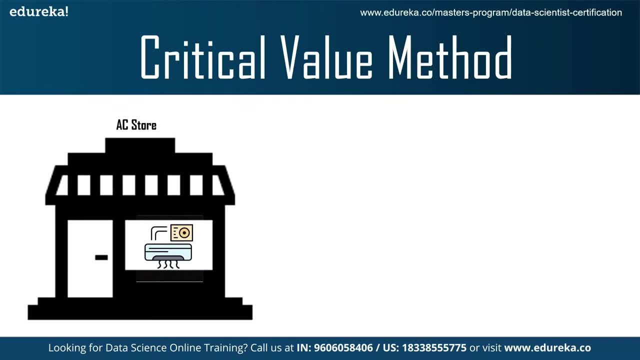 AC stores. You want to know about the mean demand of AC units per month per store during summer. Till now you have been ordering 350 AC units per store per month, based on the historic demand. but now the meteorological department has said that there will be intense heat waves, so you anticipate. 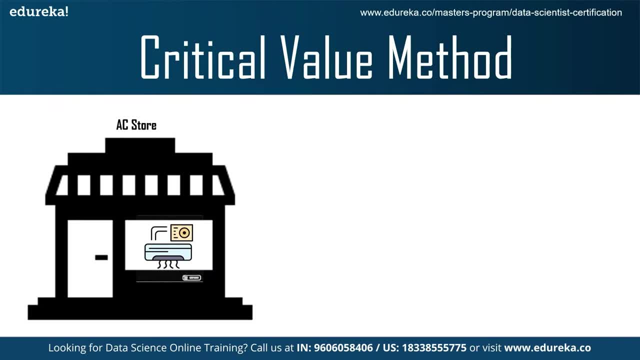 that the demand might go up. so you want to check your assumption that the average units required in one month will be different from 350 units per store. so in this case you are assuming that 350 units is the average number of units that are sold every month. when you are trying 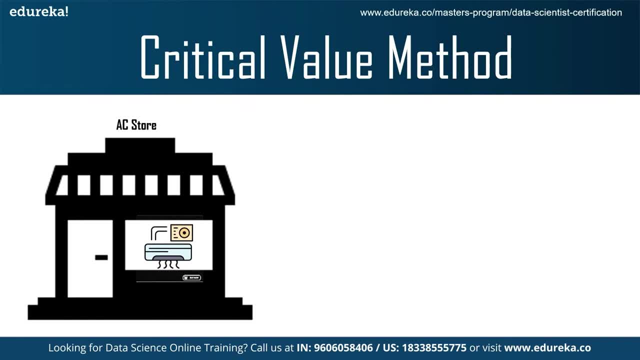 to visualize it you use a histogram and the means comes out to be 350 approximately, like you can see here. so this becomes the mean or average of population. so next you will define the null and the alternate hypothesis. you start with the null hypothesis. that is the assumption about the status quo. so you assume that H0 is true and this implies that 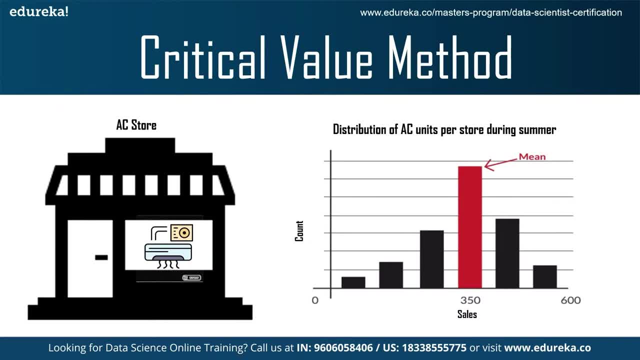 your population mean is still equal to 350. in this AC hypothesis problem, the assumption is that The mean demand for the AC units per store in one month is 350 units. so your null hypothesis H0 states that the mean demand of ACs is 350 units per store every month. as you can see, 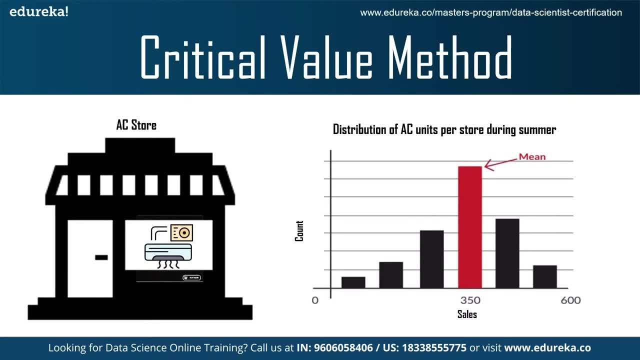 here in the graph. so now that your null hypothesis is clear, the next step is to state the alternative or research hypothesis. so H1 is the opposite of H0, which means like the opposite of null hypothesis. so it challenges the status quo. this is the assumption that you try to prove. 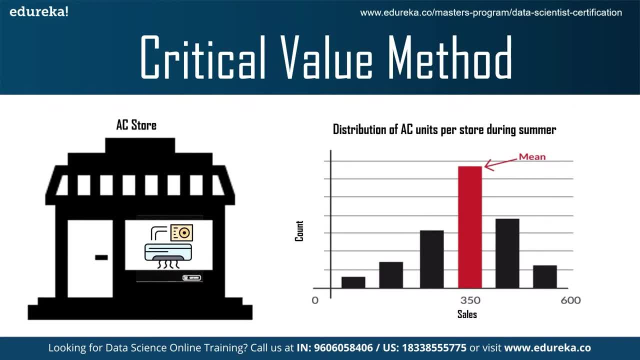 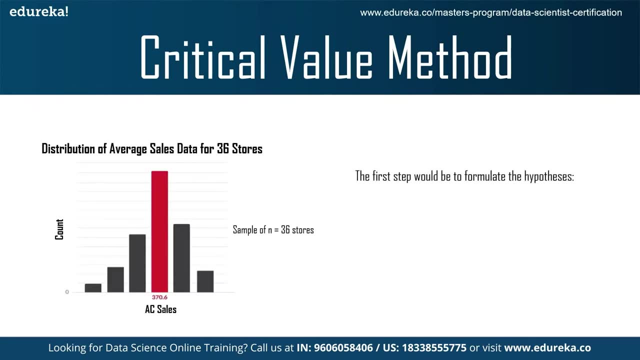 and you should examine all evidence with respect to H1. In your AC sales problem, H1 is that the population mean mu is not equals to 350. you should always examine the evidences with respect to alternative hypothesis, not with respect to null hypothesis. so now you need to formulate the hypothesis. so the first step would be to in formulating 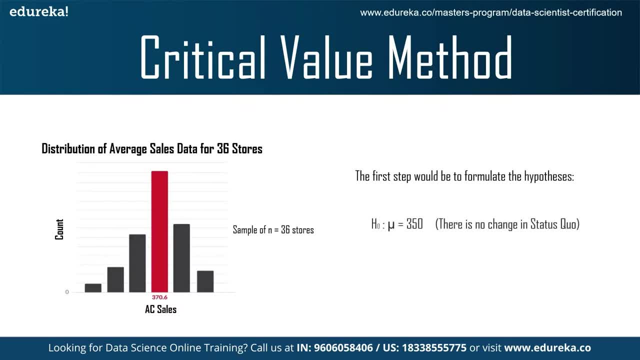 the hypothesis is that H0 is equals to 350, so there is like no change in the status quo and H1 is not equals to 350, which, as I explained you like, the status quo has changed in alternate hypothesis, Which actually is just opposite of the null hypothesis. 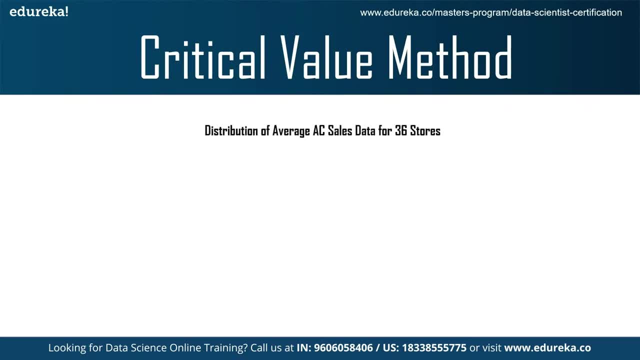 So now you need to formulate the hypothesis. so the first step would be to, in formulating the hypothesis, now you need to find the critical region for it. suppose, like, the sample mean is very far away from 350, suppose it's around 600, so you can easily say that it lies in. 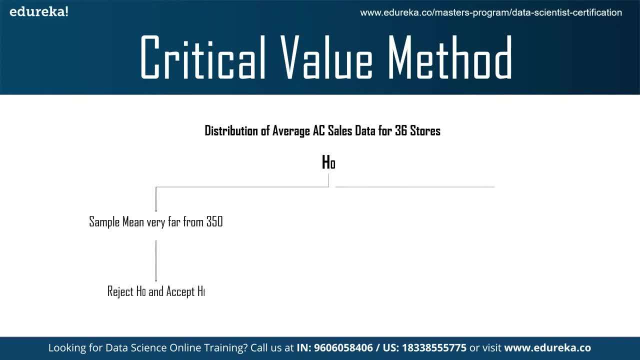 the upper critical region. and you can say, like you can easily reject the null hypothesis here and accept the alternate hypothesis, like you can say that the sales is increased and suppose sample mean is not very far away, it's like very near to the 50, like you can say: 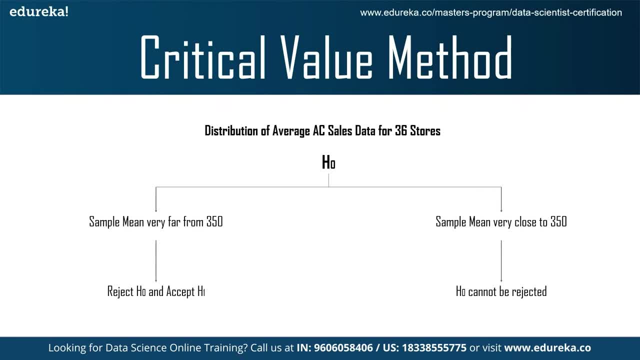 like it's around 355. if you say 355 then it's like sample mean is very close to 350. so you cannot reject the null hypothesis but you also like can't accept, because so further statistical evidence we will see for it and then we will decide what we need to go for. 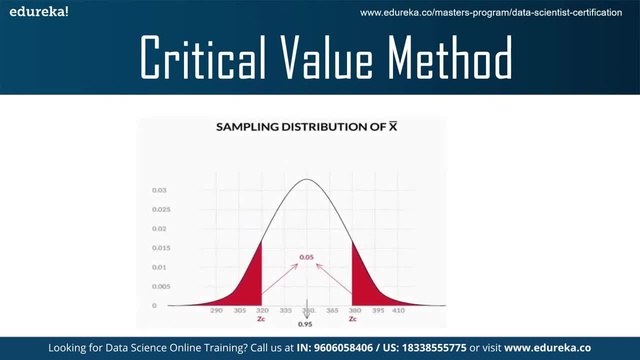 so for that we need to do the sampling distribution of the X bar. so as you're working on samples, you will compute the standard error. the standard error can be calculated as standard deviation by square root of number of samples. so you calculate the standard error because you want. 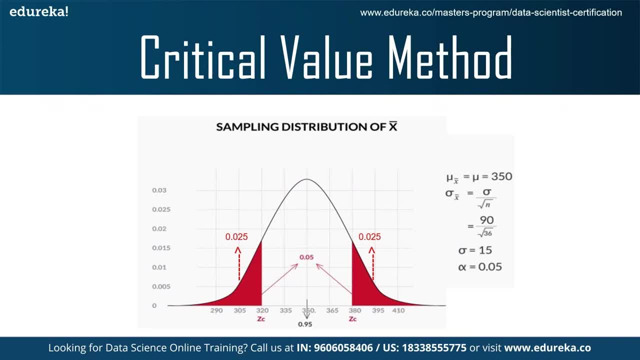 to know is the value 370.16 has significant distance from the mean 350.. So you need to calculate the standard error So the null hypothesis can be rejected. Now we have the normal distribution of sample means for the mean of 350 and we have the 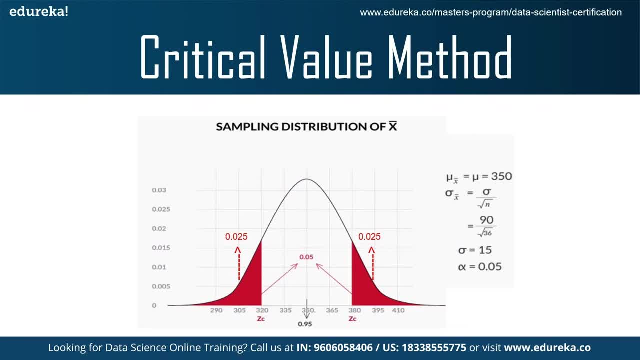 standard error, or we can say that sample standard deviation, which is 15.. So now we have to find the critical value through it. so to find the critical value, you need to first specify the probability of an error happening and we need to like, keep this in mind: the probability of an error happening should be the least. 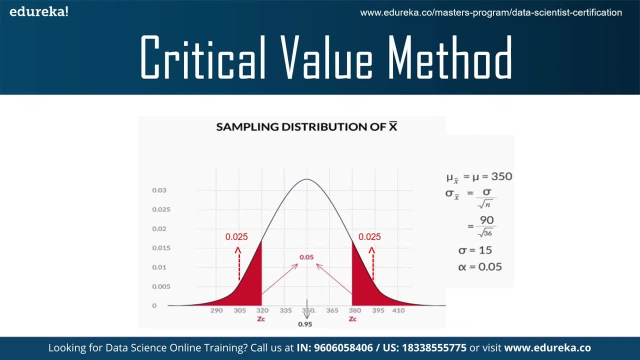 So suppose you find out the critical value to be 380. So it's like if you get the sales of more than 380, you can easily reject the null hypothesis. So we can take the significance error value, that is alpha, to be 0.05, which is normally. 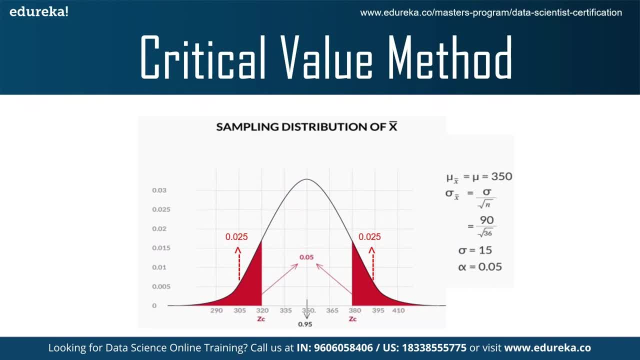 taken as 0.05 only. So we can say through this that the percentage of error happening is 5% only. for 95% of the time the condition will be right means like for 5% of the case when the you will reject. 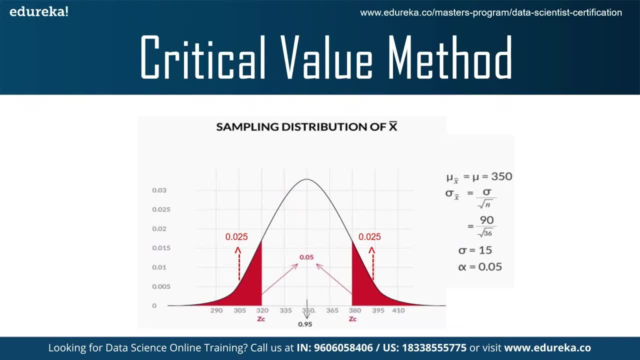 the null hypothesis when null hypothesis will be actually true and for 95% of the cases that will be acceptance reason. So it's like we fail to reject the null hypothesis in 95% of the cases when it is actually true, So the error won't take place in 95% of the time. 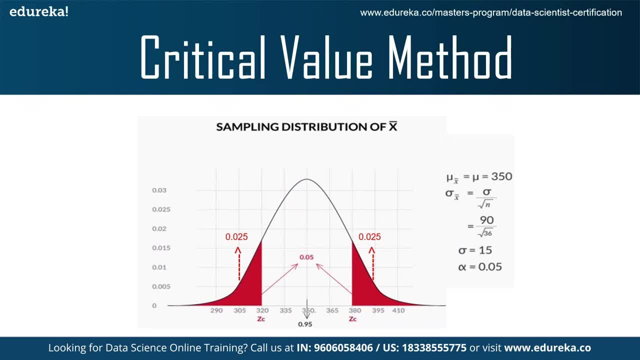 So here you can see like there is a lower critical region, upper critical region. there is a ZC value we have to find out for it. So as it's, 5% means 0.05, so that will be like divided into half for lower critical region. 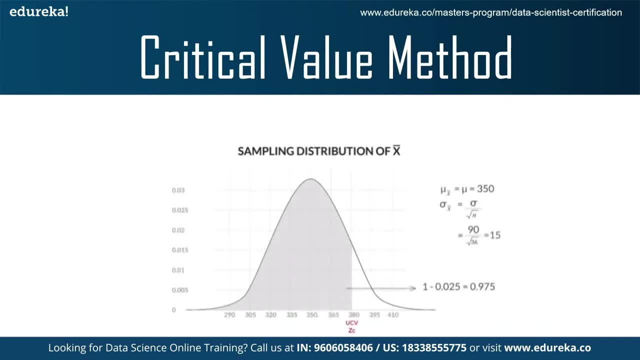 and for half for upper critical region. So for upper critical value, you find it by subtracting it from 1 for area under this curve, which comes out to be 0.95.. So for upper critical value, you find it by subtracting it from 1 for area under this. 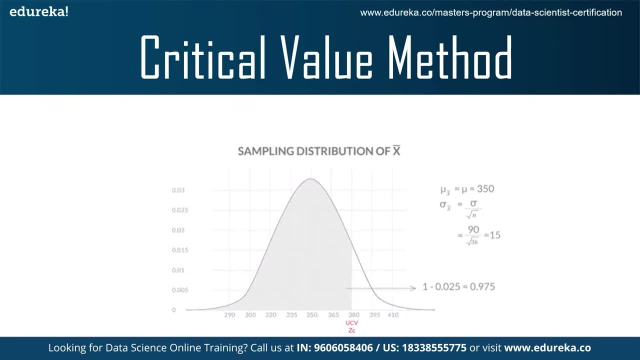 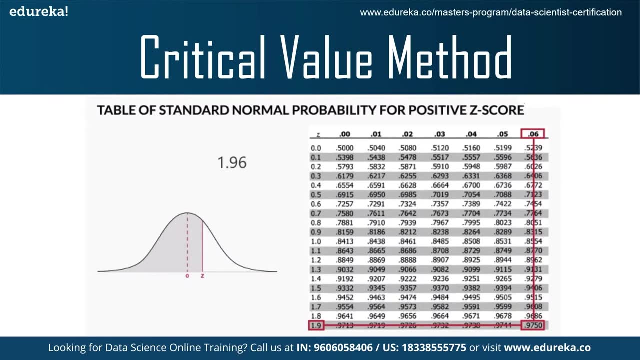 curve which comes out to be 0.95.. Then we have to find the Zscore for it. that can be found out through the table. If you see horizontally and vertically: 0.9750. horizontally it is 1.9 and vertically it is. 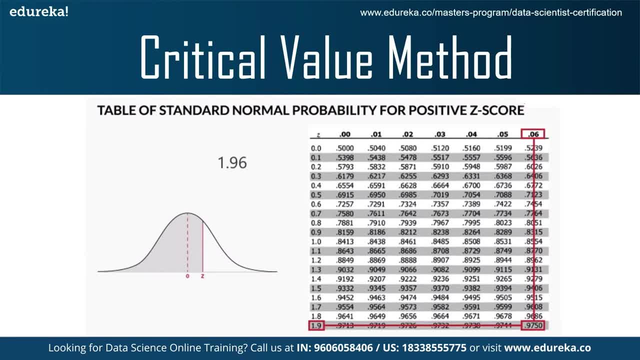 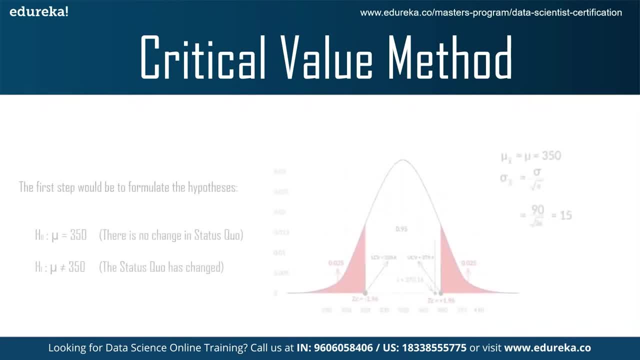 0.06. if you add it comes out to be 1.96.. So then you calculate the critical value like upper critical value and lower critical value from the value of ZC, So that you can calculate through this formula like: critical value equals to mu plus Zscore. 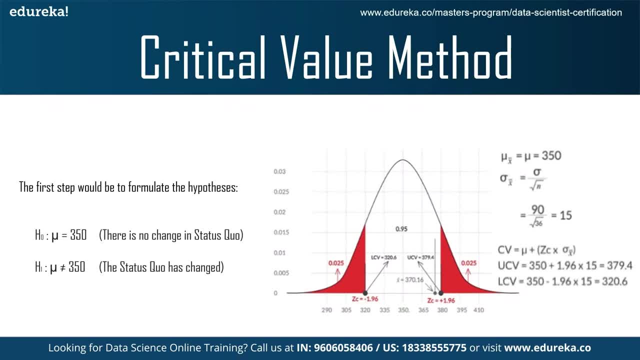 into standard deviation of the sample. Okay, So you can see like upper critical value comes out to be 379.4, which is under the acceptance region, and LCV comes out to be 320.6.. So, as you can see, like the sample mean is less than upper critical. 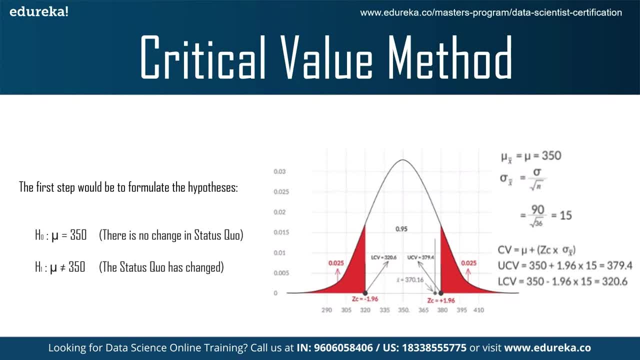 value and greater than lower critical value, that is, it is in the acceptance region. So the final decision is that we fail to reject the null hypothesis means null hypothesis is true, So we can say that sales will be like equivalent to 350.. So now let's understand in a standard form. 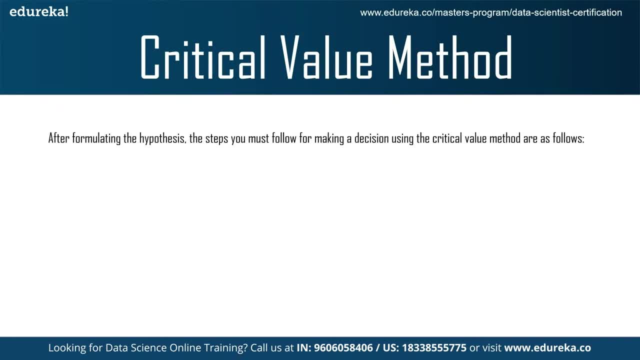 like the critical value methods. So, after formulating the hypothesis, the steps you must follow for making a decision using the critical value methods are as follows. You can see like you have to calculate the value of z score from the given value of alpha means: significance level. 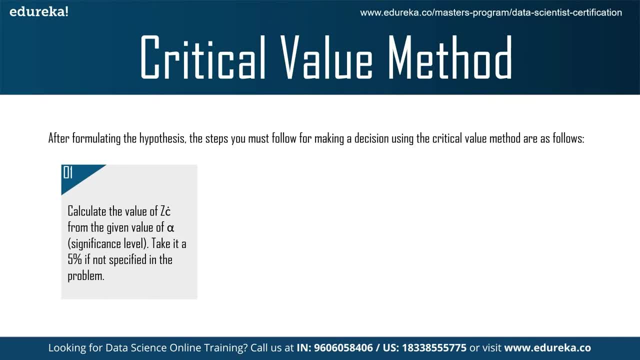 which we have taken as 0.05.. So, like you can see, like 0.05 is given, as 5% is not specified in the problem. So then you have to calculate critical values like upper critical value and lower critical value from the value of zc, and finally make the decision on the basis of the value of. 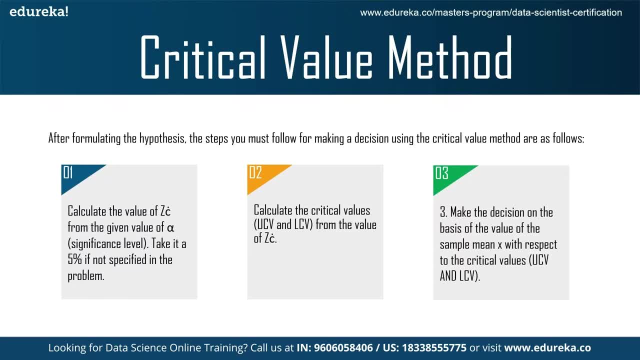 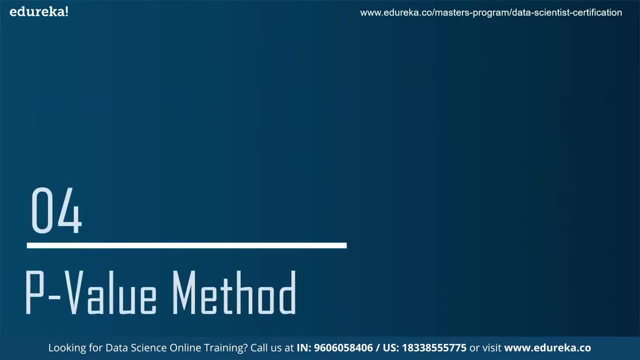 the sample mean x with respect to the critical value. I hope this made you understand the critical value method. So, apart from critical value method, there's other methods as well to reject the null hypothesis or failing to reject the null hypothesis. So we will look at one of these methods, which is p-value method. So we will now find the p-value. 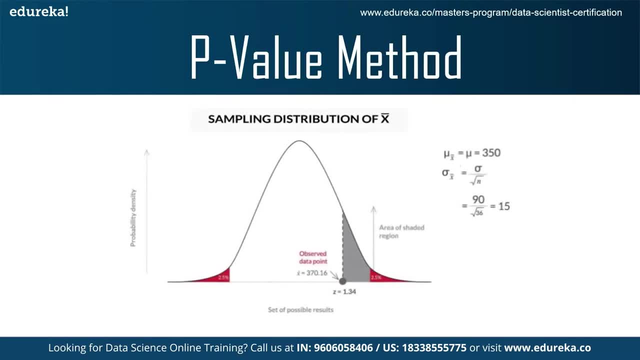 for the same AC sales example. So you can see the p-value is the shaded region from the gray area region. So we have to find the like for the 70.16 of mean p-value will be like for like greater than 370.16.. So we need to find the p-value for the z score: 1.34.. So if we look for z table you can see. 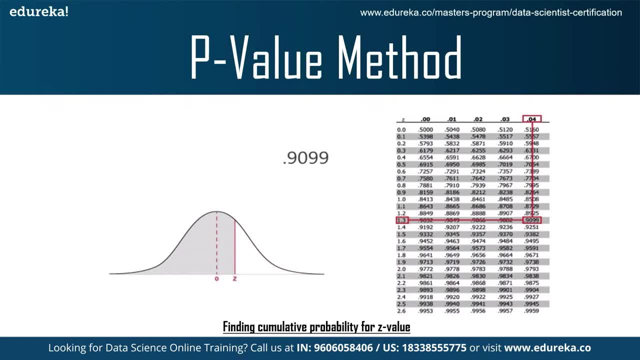 like, the value will be for 0.9099.. You can see how horizontally it has been plotted and how vertically it has been plotted for 1.3 and 0.04.. We have find the value to be 0.9099.. So now for 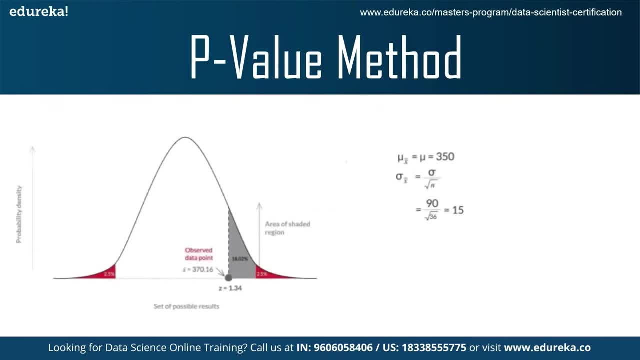 calculating the p-value, we will subtract 0.9099 from 1.. So it will come out to be 0.0901, and just a two-tailed test. So we will multiply it by 2 and we get the value as 0.1802, that is, 18.02%. 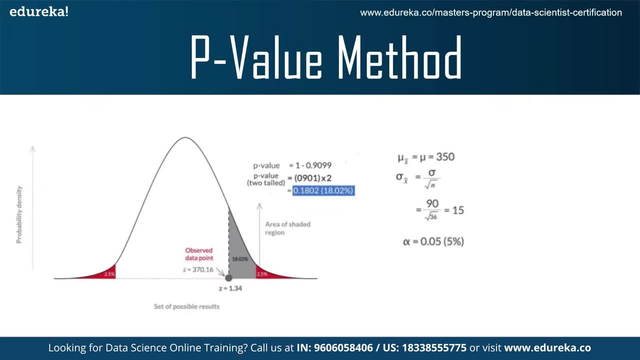 And now. so if you see the significance level, which was 0.05, that is 5%. So you can see like p-value is higher than the significance level. So we can now easily say that we cannot reject the null hypothesis. So the final decision is that we fail to reject the null hypothesis. So after: 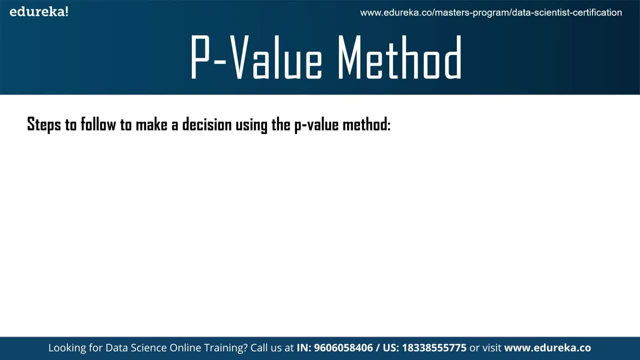 formulating the null and alternate hypothesis. the steps to follow in order to making a decision using the p-value method, like we have understood in the process, is that we have to calculate the value of the z-score for the sample mean point on the distribution. Then we need to calculate the 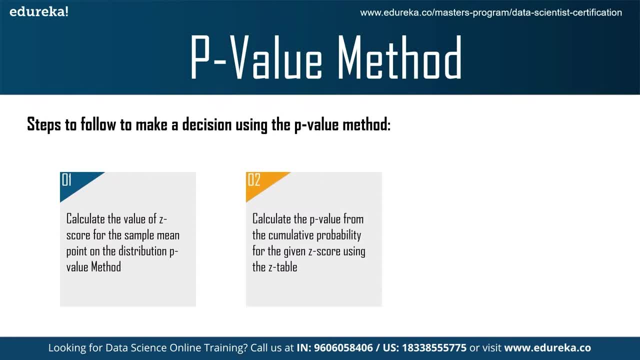 p-value from the cumulative probability for the given z-score using the z-table. So, and the third step is to finally make a decision on the basis of the p-value like. multiply it by 2 for a two-tailed test with respect to the given value of alpha means the significance value. So by comparing, 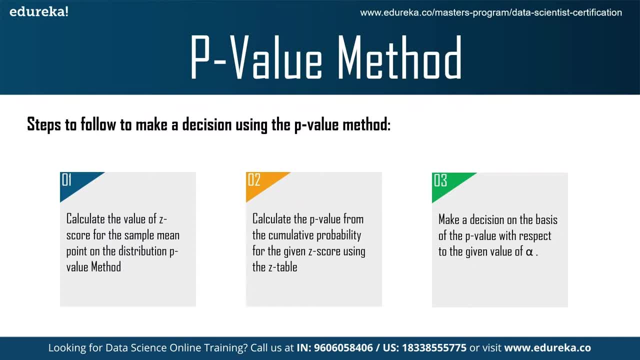 that we have reached the final conclusion. I hope this made you understand that in the p-value method as well, how we can use it for rejecting null hypothesis and for failing to reject the hypothesis. Now let's understand the types of errors in hypothesis testing which can occur. So 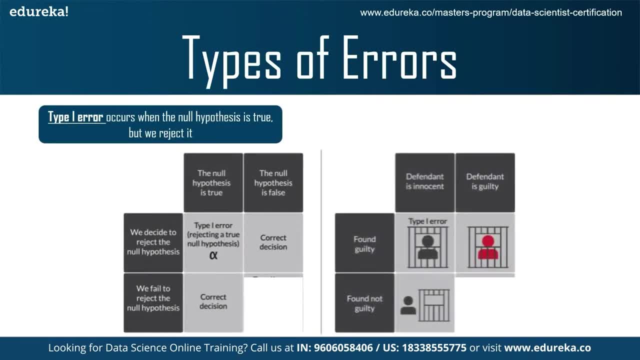 the first type of error which can occur in hypothesis testing- we call it as type 1 error- which occurs when the null hypothesis is actually true and we reject it. So if you remember the criminal trial example, so we need to have all amount of concrete evidences to prove that accused. 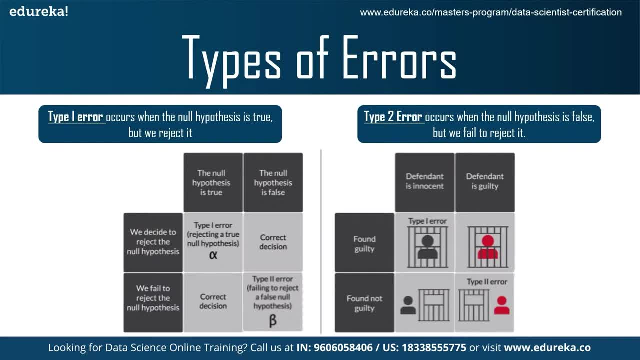 has actually done the crime. Suppose judgment for the crime is a death penalty, just suppose. and if he gives the proper evidences and he gives the judgment as a death penalty and somehow, like those evidences doesn't prove that he is accused, and suppose in reality the accused is actually. 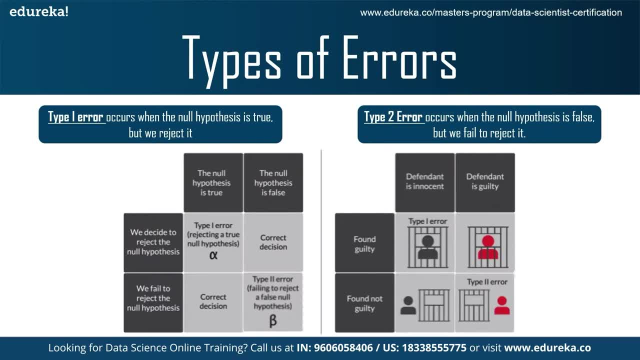 innocent and he gets the death penalty. that will be a very big error so which can actually affect the society a lot. So that's the- I mean, say, the density of type 1 error. So we need to keep that in mind, that we need to have concrete evidences to support our alternate hypothesis so we don't 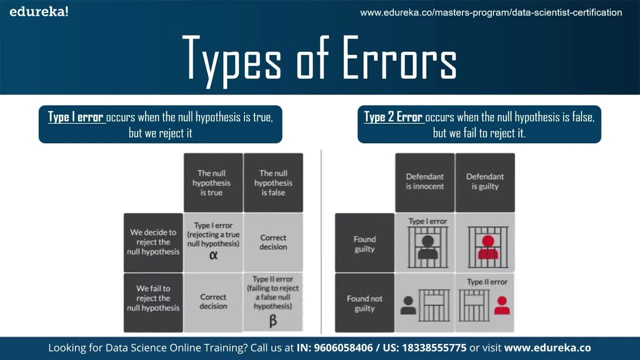 have to reject null hypothesis like that, we need to have proper, concrete evidences For it. so then there is a second kind of error, which is a type 2 error, which occurs when the null hypothesis is actually false, but we still fail to reject it. So like type 1, error is denoted. 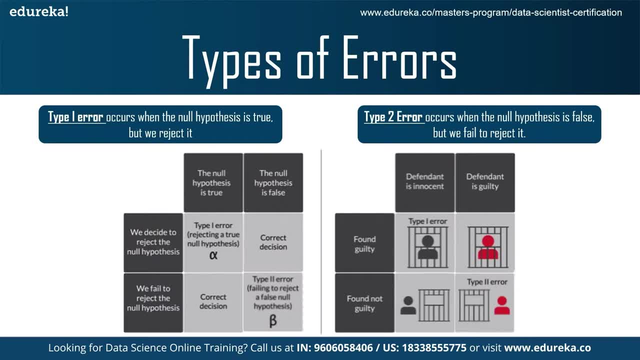 by alpha and the type 2 error is being denoted by beta. So in the same criminal trial example, suppose the accused has actually done the crime. he is actually a criminal, but we don't have enough evidences to prove that he has done the crime. So that will lead to type 2 error, because that 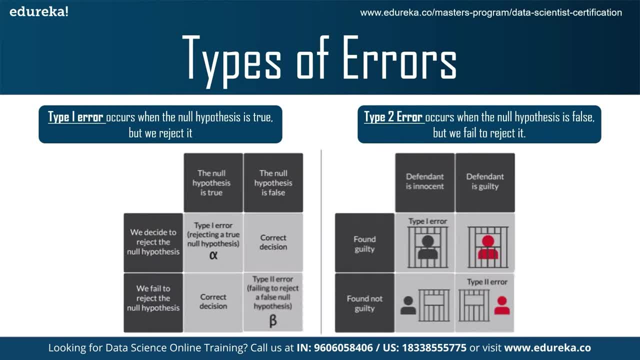 person can actually, like the criminal, can actually again go and do several other crimes and which can be harmful for the society. That is also like a very grave situation. So these are, you can say, the types of error which can take place in hypothesis testing: type 1 and type 2 error. I hope you have understood this concept of errors as well. 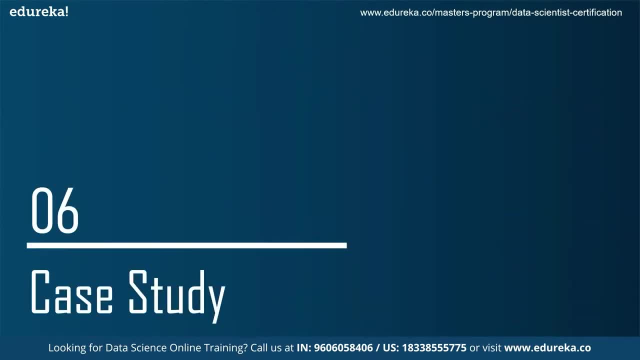 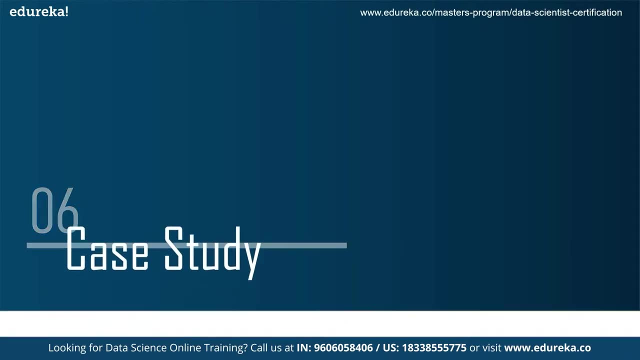 So now that you have a conceptual understanding of hypothesis testing, let's see a case study of Flipkart and how hypothesis testing can be applied in like real-time business and e-commerce business. So let's first have a business understanding and understand the problem statement as well. 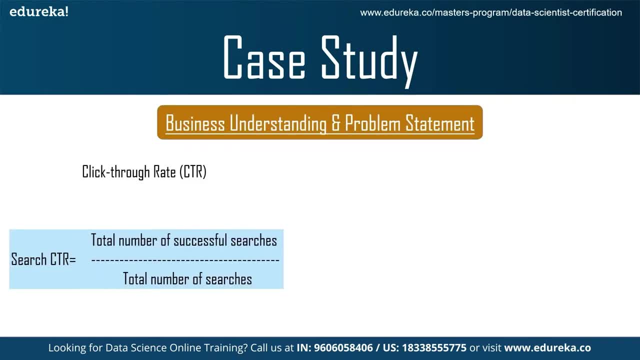 So in this entire demonstration, you will be looking at an important business metric used in the e-commerce industry, that is, the click-through rate, popularly known as CTR. So this is a very important business metric, especially for the businesses that have a website presence or a application presence, So on. 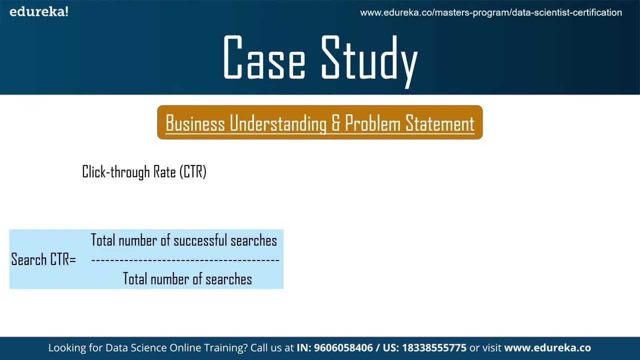 this metric, we will be making claims and hypothesis and then test them using the concepts that we learned previously. Before getting into hypothesis testing part, let's understand what CTR means and how specifically we are like going to use it in this demonstration. So click-through rate is a. 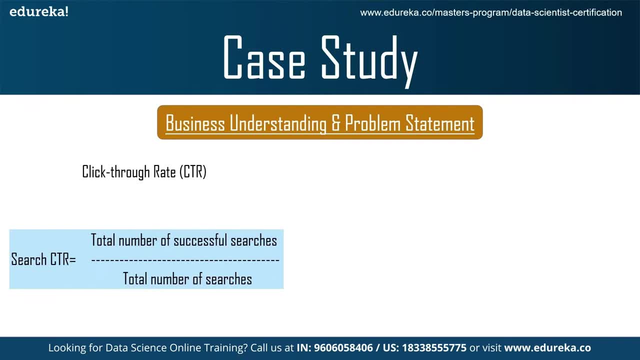 generic yet important term in the online marketing industry. In plain terms, it measures the action rate of some entity, May it be a banner ad or a like, a home page for some website. or we can say, if there's an ad tech website, so like if people will be opening a certain course and applying for 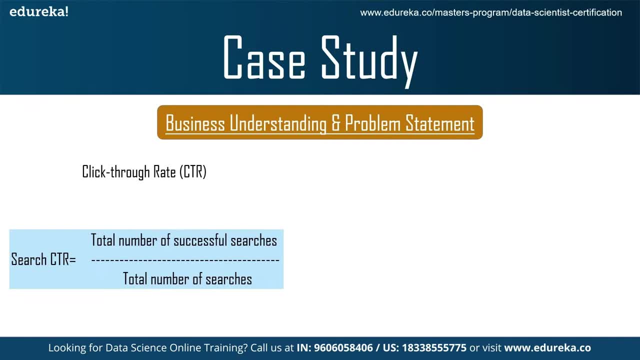 it. So those are like action rate of that course, of that entity. So now let's understand how the search through rate, or CTR, can be defined in the search context. So in the case of online search, the CTR is the proportion of search content. So, in the case of online search, the CTR is the proportion of 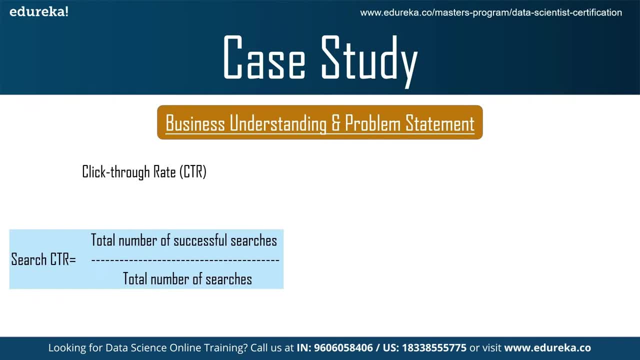 searches that was successful. when you are trying to compute the search CTR, The relevant formula for it can be given as like total number of successful searches by total number of searches. So what are the successful searches? So I will give you an example for search CTR through Flipkart only. 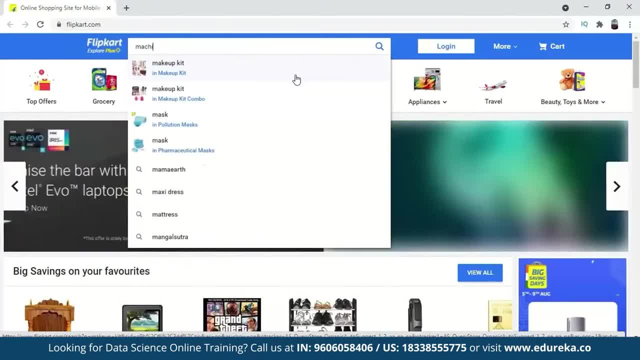 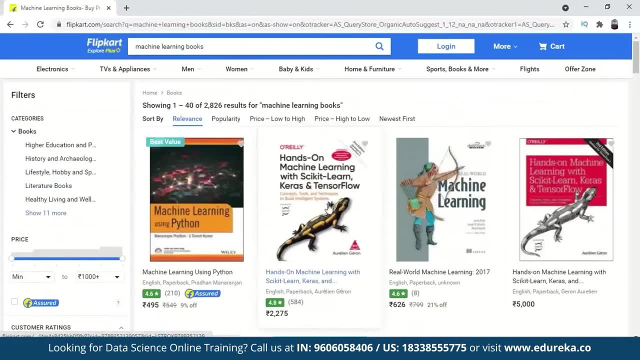 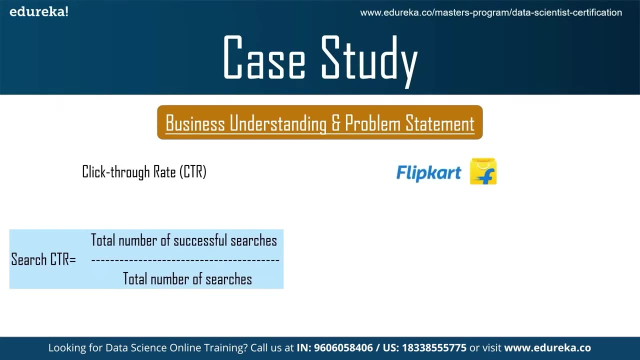 So if you search for like, we can search for machine learning books. This is the like normal search we are doing and these are the results. and if I go open a particular search into it, so that becomes a search. So now let's get introduced to the industry problem statement that we are going to. 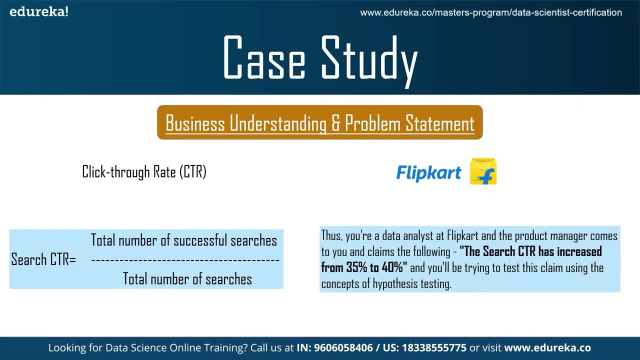 solve in this entire case study. So suppose that you are a data analyst at Flipkart and you works with a product manager and that product manager claim that the search CTR has increased from 35% to 40%, and you will be trying to test this claim using the concepts of hypothesis testing. So let's. 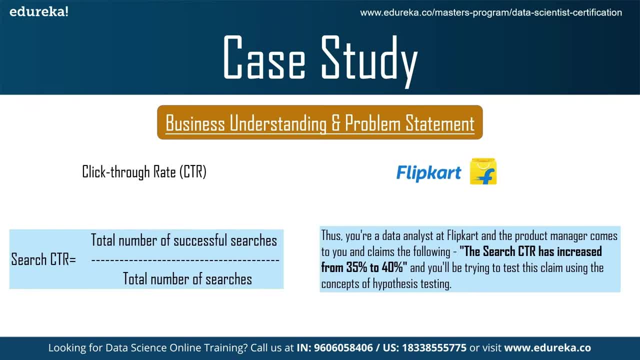 dissect the problem statement a bit further, which will help us in hypothesis formulation as well. So to summarize this problem statement, you can say that the product manager is like claiming that the average population search CTR is 40%. That means, out of 100 such searches on Flipkart website, around 40 searches will like result in conversions. means 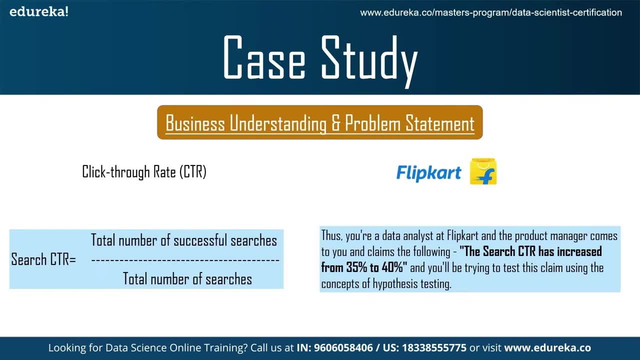 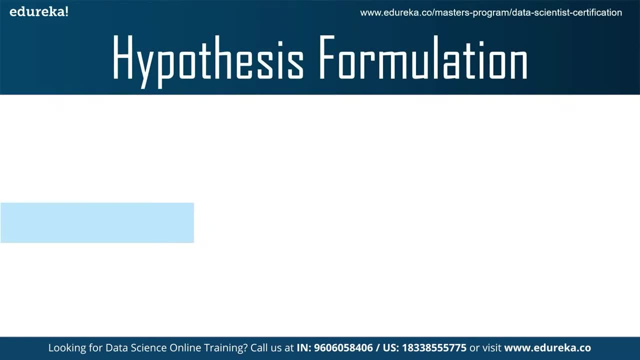 in successful searches. So using this we can like formulate: the hypothesis means null and alternate hypothesis. So, according to the giving claim, as the search rate is 40%, which means null hypothesis, will be 0.4 and the alternate hypothesis, which means we are going to challenge the claim. So the 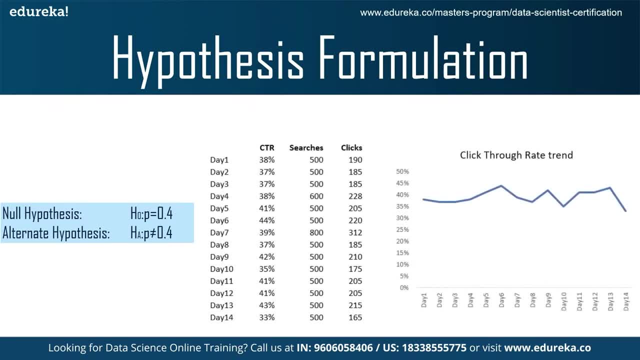 data is like P0 equals to 0.4.. Now we have taken this data of 14 days. It's like a sample we can say, and in this we can say like on day one it has like 38% and 37% day two, and. but on some days we have 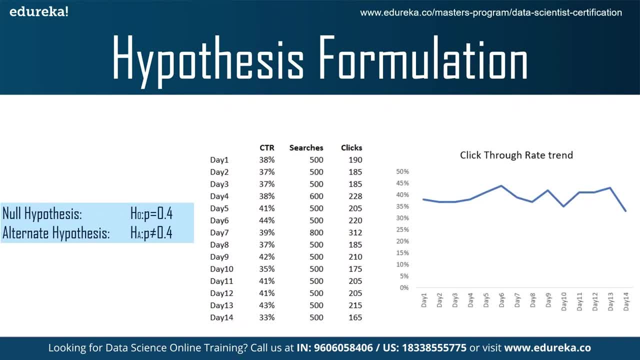 44% as well, 43%, 41% as well. So for the 14 days data we have taken for the formulation for further like backing up our research hypothesis. So now you must be thinking we can like go ahead and conduct the hypothesis test directly on the given data. but think about it for a while, Like which. 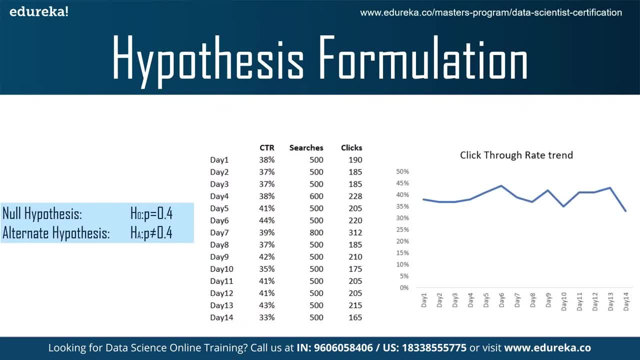 exactly are you going to test the hypothesis on? Is it the CTR of one day, one week or multiple days, Since the data is varying a lot across all days? how do we ensure that the sample is a random representation one, Because we need to have an appropriate representative sample. Let's understand. 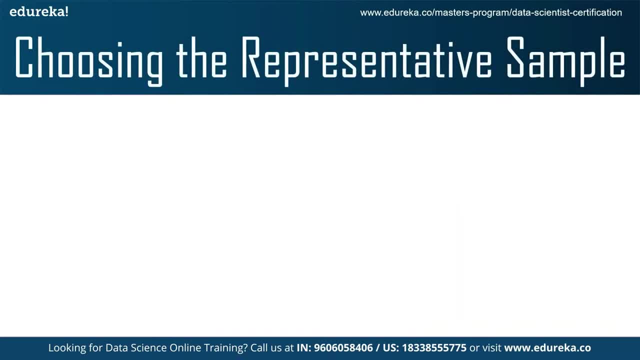 how to choose the representative sample. So do you think like we need to take the data in a manner like it should show like 40% CTR rate on every day? That's not possible, right? That's not happening. So we will, of course, take the data where like. 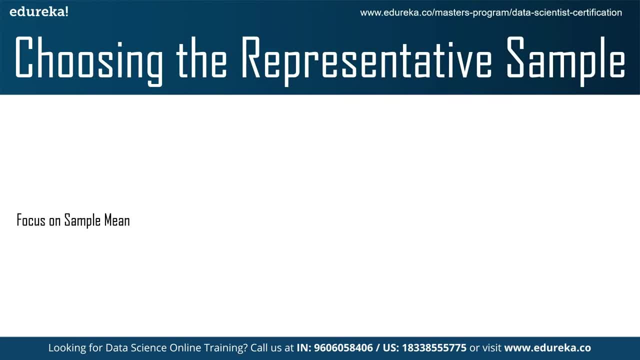 on some days there will be like 40% CTR rate there, on some day 35%, there may be some day 45% and it will vary somewhat On weekday, it will vary on weekends, it will vary right. So according to given blame, population mean for the given search, CTR is 40% or we can say 0.4.. 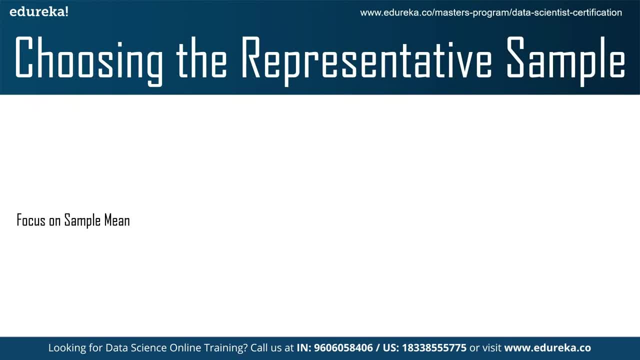 Now the sample we have seen can show variation and may not be exactly equal to the value that is 40%. So it is only that, on an average, when you compute the mean CTR for several days, that will bring the result. 0.4 means 40%. So now, once you have understood this concept, you need to know which. 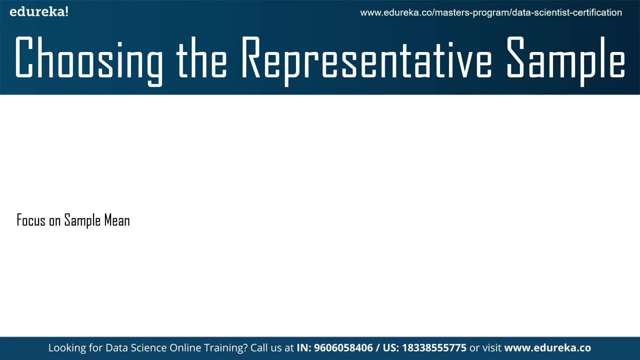 distribution you need to look at So like: do you need to see the population distribution or sample distribution means some different samples. So now that we have understood that we have to focus on sample mean, we will finally compute the sample parameters for the given sample data. So we see. 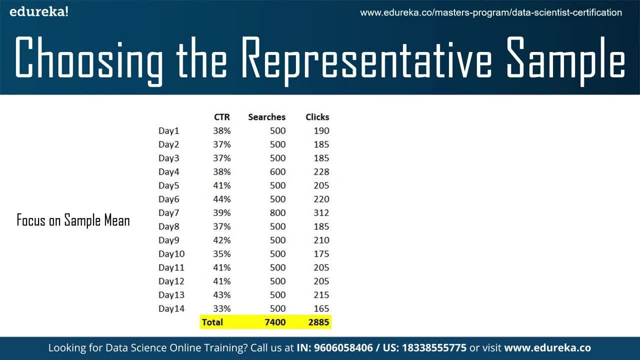 that like we can see the CTR, it's varying and we see like for every day. there are like normal searches which happen around 500- 500 we can see for days. So we can see that like we can see the one day 2, and then on some day it happens to be 600, some day it happens to be 800. So it's like that. 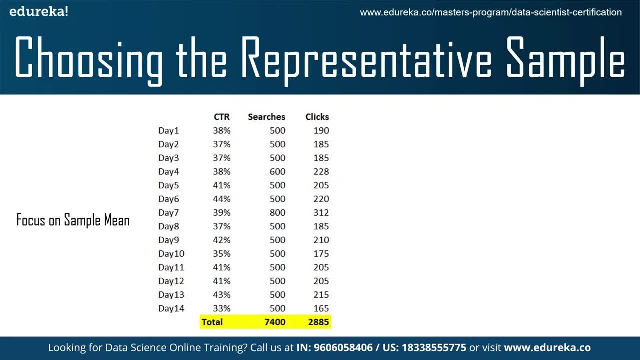 So we can see here the clicks as well. The successful clicks means we can see successful searches. Those are 190, 185. on some days it is 2312, 175 as well. So we can see the total searches like 7400 and clicks come out to be 2885.. So for the 14 days, come out with the average search CTR. 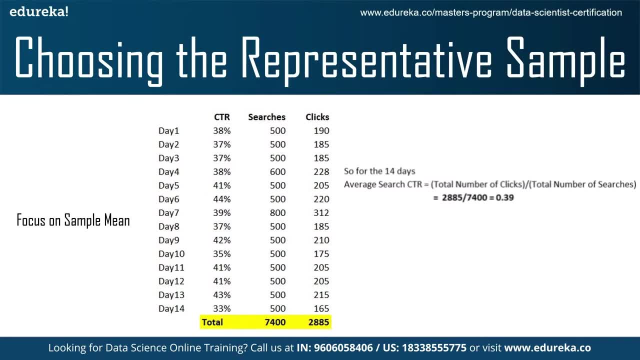 that is the total number of clicks out of total number of searches, So which results in 0.39 as the average search CTR. Therefore, like we can say, the sample mean comes out to be 0.39 and sample size is 7400.. So we can. 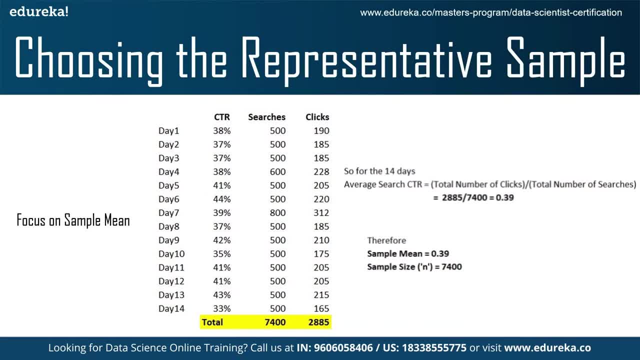 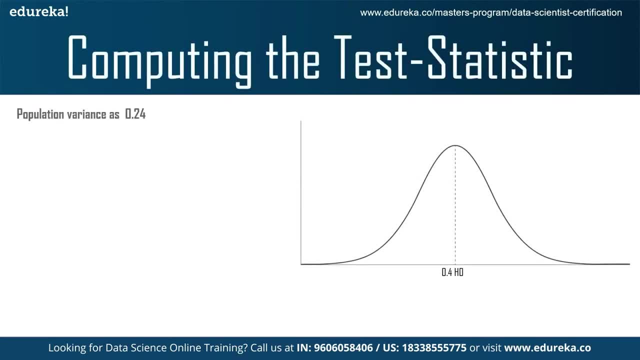 say that we have taken a sample of a total searches of 7400.. So that brings the sample size to 7400.. So next step is we need to compute the test statistic. So now that we have the required sample parameters, we need to compute the test statistic for the given sample. For this we need 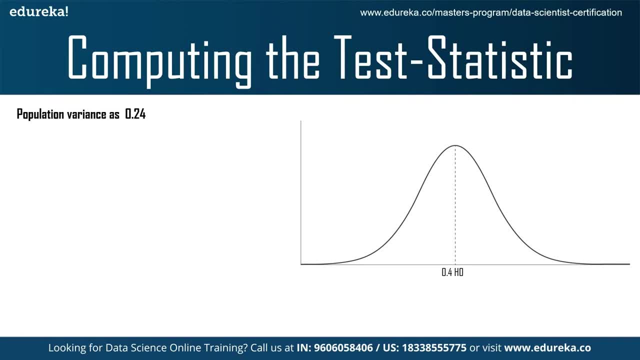 the sampling distribution standard deviation as well. So let's say you are given the population variance of 0.24.. Now let's go ahead and compute the sampling distributions, standard version. Note that you are already given the population variance of 0.24.. So from this and the given sample size, 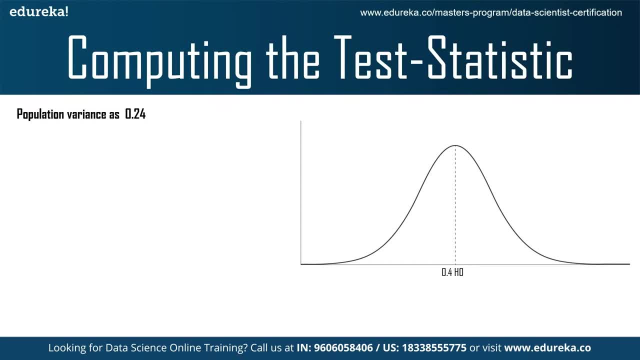 you need to compute the sampling distribution standard deviation. Recall that from the center limit theorem the formula for sample distributions, standard deviations, comes out to be sigma by root n. So we can say that sigma square, which is population variance, is 0.24 and as we have, 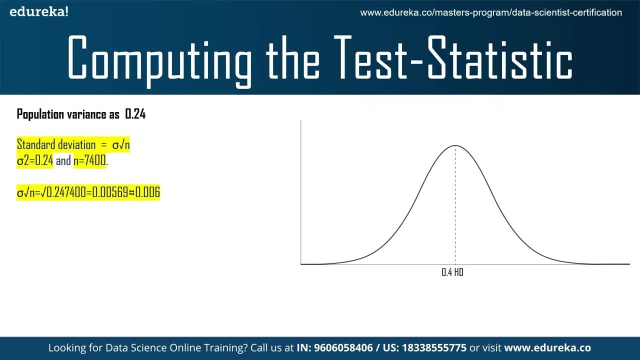 already found out, the sample size, that is n, equals to 7400.. The sampling distribution standard deviation is computed as sigma by root n, which comes out to be 0.006.. So that we have calculated the sampling distribution standard deviation. given from central limit theorem comes out to be 0.006.. So now let's go ahead and calculate the test statistic. 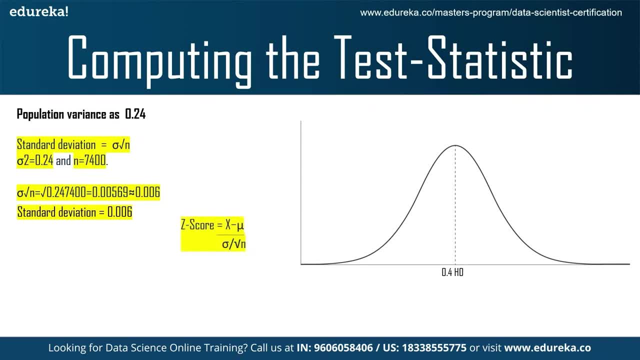 for the sample, which you know will be its z score. So z score, as you know like, can be calculated by the following formula, that is, x minus mu, by sigma, by root n. Now for the gain problem. we have the sampling distribution, standard deviation as follows: we can say: like sample mean is 0.39. 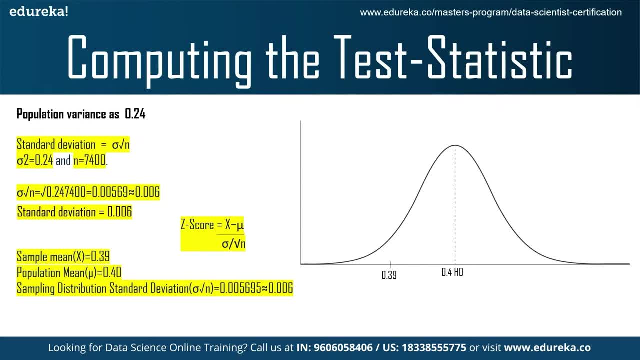 population mean is 0.40. that is claimed by the project manager as well. and sampling distribution like standard deviation, we have got 0.006.. So substituting the values we get like in the formula, that is, x, we have 0.39, mu is 0.40 and sigma value is 0.005 means 0.006.. We can see the sigma by root. 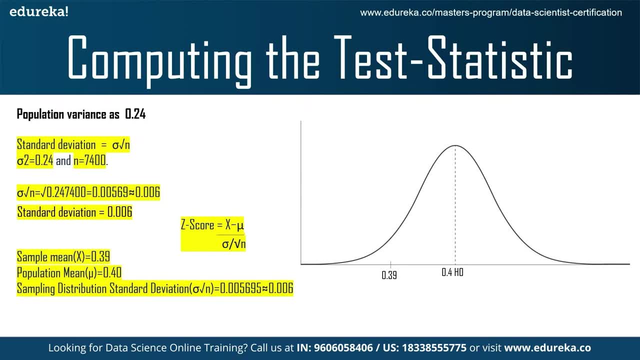 n value, that is the sampling distribution standard deviation, which is 0.006, and we get this value as z value, that is 1.75.. So this is the test statistic of our sample data. Next method is we have to find the critical region. 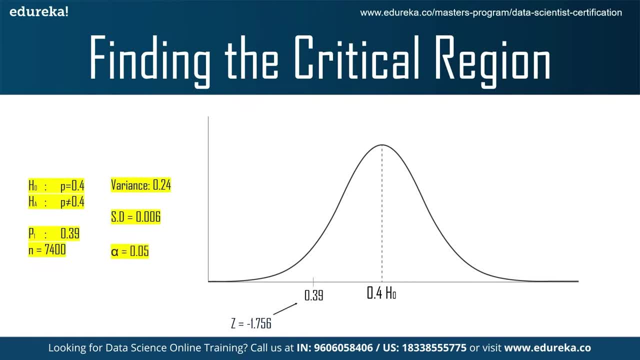 and we already know like what is alternate and null hypothesis, as well as the population variance that is 0.24, as well as the sample mean to be 0.39 and sample size to be 7400.. That is what we got from the test statistics, from our sample data. Second crucial parameter that we need is the level. 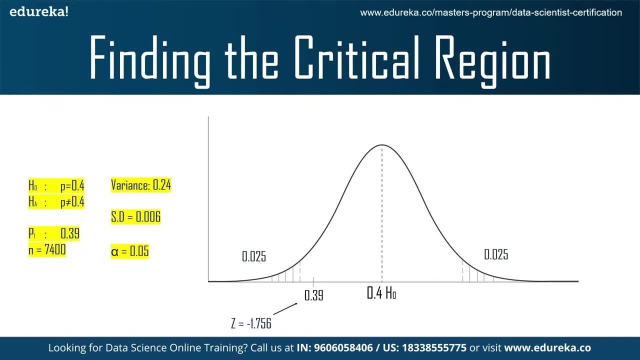 of significance of alpha. that is like how much the results can deviate. So the level of confidence that we can get from the test is the permissible limit to which the sample can deviate and for the given test we can take it as 0.05.. It is like a industry thumb rule, we can say, like taking the 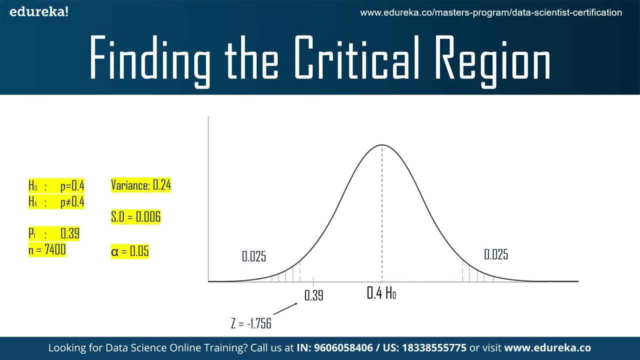 alpha value to be 0.05. but sometimes if you have other situations and conditions that are different from them, then you can have a different like alpha value as well. but here we do not have any such conditions, situations which can affect our significance level. So we have just taken it as 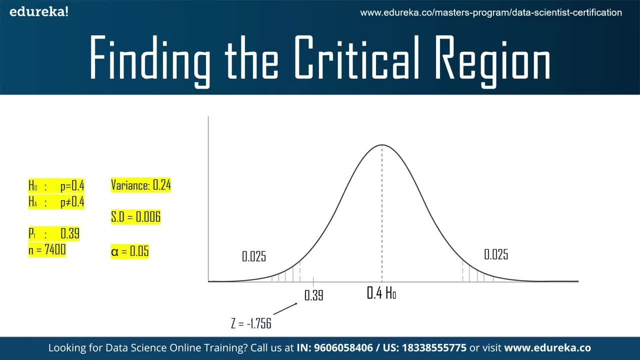 0.05.. So using this, we can find the critical region for the given test conditions. So for finding the critical region, you need to use the like value of alpha means, the significance level, as well as the given null hypothesis as well, Since it is a two-tailed test, so we need to have a cut-off range. 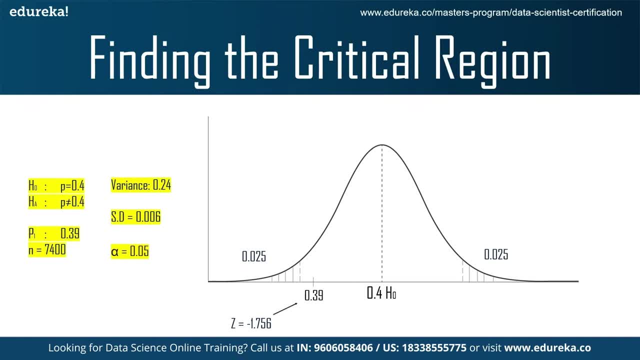 as well. So this cut-off range will be divided into two. So as we have 0.05 as the significance level, that will be divided into two. So that will bring us two like regions on the left side and the right side. that will be lower critical value and upper critical value. So that will be divided into. 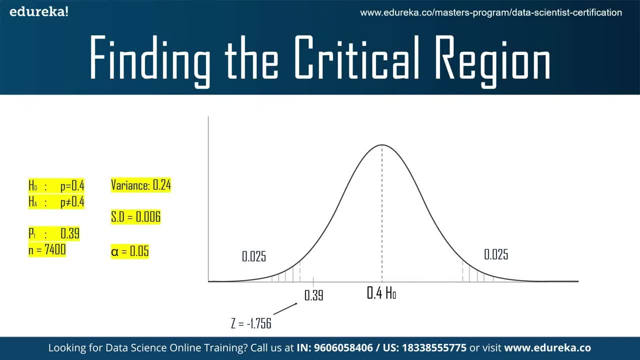 two by alpha, So that will comes out to be 0.025.. So that will come out to be 0.025.. So that will be divided into two by alpha. So if your value comes under 0.025 on the left side or the right, 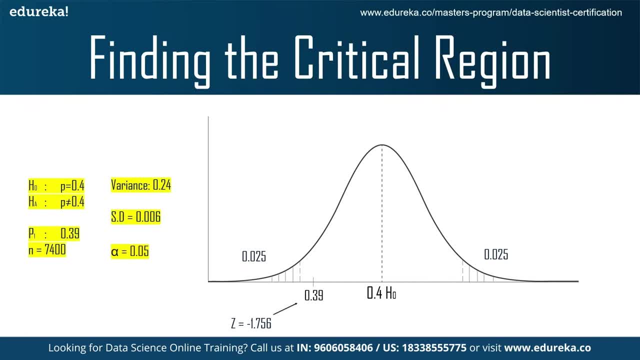 side, then we can like reject the null hypothesis. But as we saw that our value- 0.39, like that- comes out to be 1 minus 1.756, that doesn't come under the critical region, So it's like become easier for us to make the final decision based on the given hypothesis. So now that you have found the 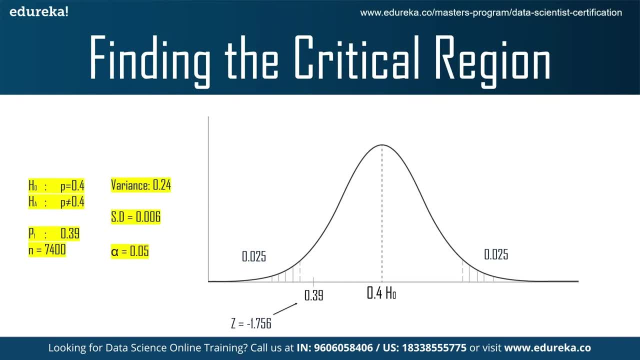 critical region, you need to check where your test statistic lies and based on that, make the decision. So on the basis of our evaluation of critical region and on the basis of z-score and everything, we have found that we can't reject the null hypothesis. So therefore we can say that we haven't found enough statistical evidence to disprove the 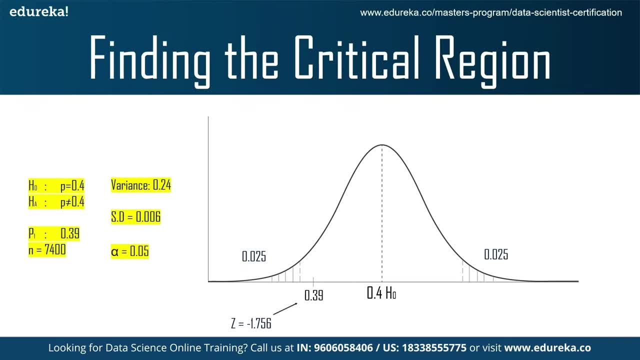 product manager's claim. So this is about the finding the critical region. And now, other than finding the critical region, we have another approach, which is the p-value approach, to do the same as well. So let's go ahead and use that approach as well. So here, 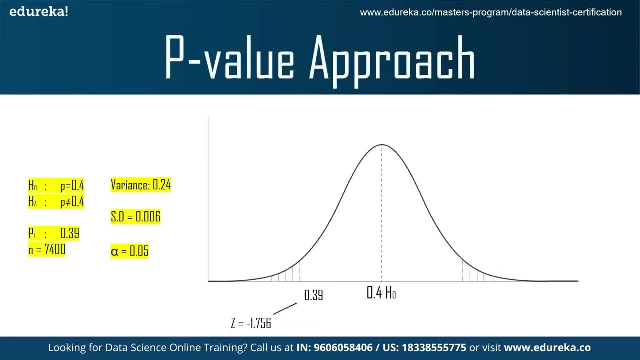 you will be doing the same hypothesis using an alternative procedure, that is, the p-value approach. So this is the most common way of finding the significance of test results in the industry. So, technically like, p-value is the probability of observing values which are similar to more. 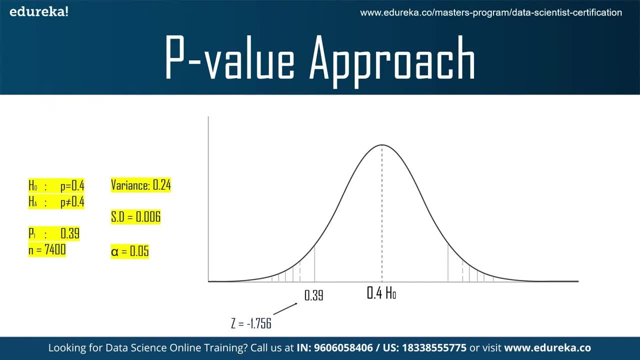 extreme than the observed value, given that the null hypothesis is true. This metric also enables us to determine whether the given test statistic gives us sufficient evidence to reject or fail to reject the null hypothesis. So let's go ahead and use this approach as well. So, when you compute, 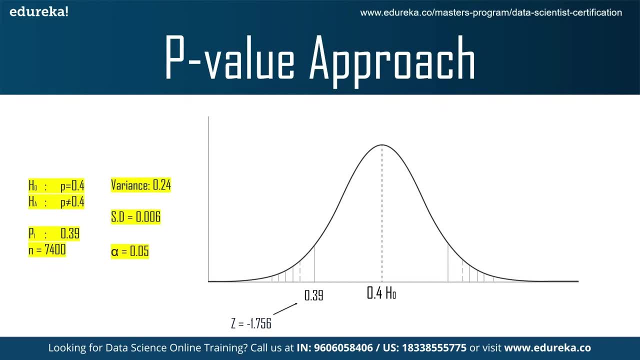 the p-value, you sort of followed an opposite route to the original critical value route. So as we know that p-value approach is more extreme approach of getting the sufficient evidence for rejecting or failing to reject the null hypothesis, So on that basis we can get more extreme limits. 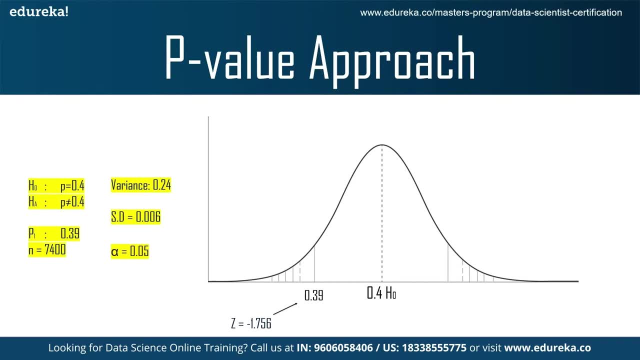 So we can get it like here for 0.39 and similarly on the right side as well. On the left and right side we have got more extreme limits, So now we can like compute the p-value. So for computing the probability corresponding to the given z square, it is minus 1.756.. We get the p-value as 0.039.. 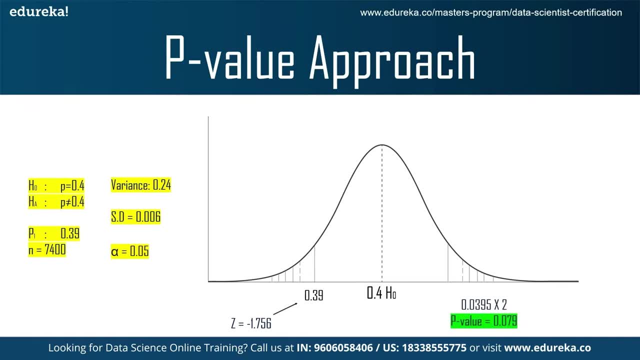 Since this is a two-tailed test, you multiply this value with the 2 and you obtain the p-value as 0.079.. Now, since the value is greater than the given level of significance, you fail to reject the null hypothesis. To summarize, the p-value approach also gives us the 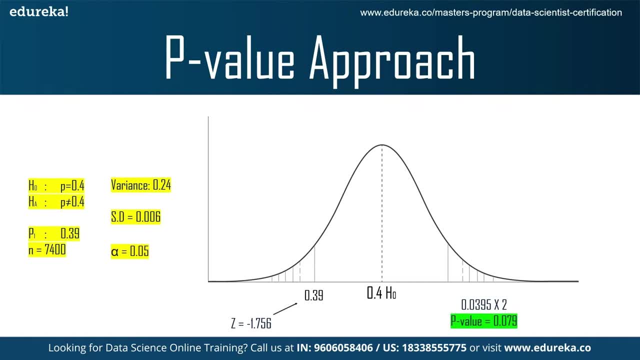 same result as the critical value approach, which is that either both will reject the null hypothesis or fail to reject the null hypothesis. So with this we come to the same conclusion as of critical value approach: that we have still don't have a proper evidences like proper, sufficient evidences. 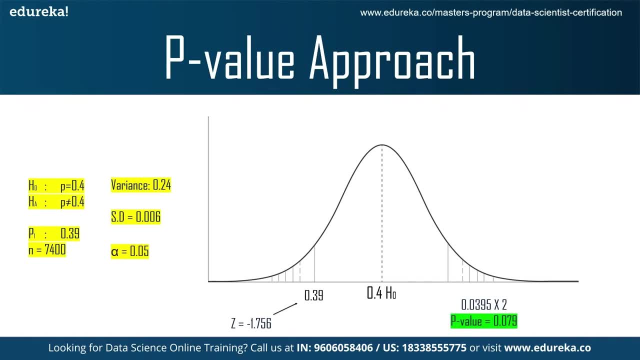 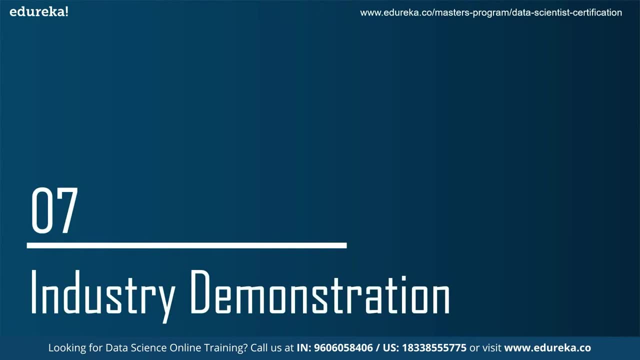 to reject the project manager's claims of click-through rate. Now that we have learned about the basic concepts of hypothesis testing and we have learned like how to formulate the hypothesis and then make a decision through either the critical value method or through the p-value method, So we will now learn how. 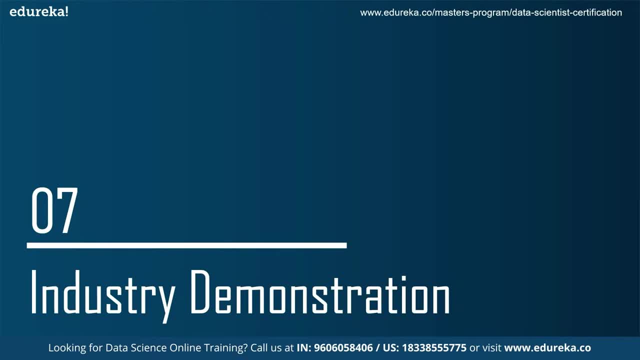 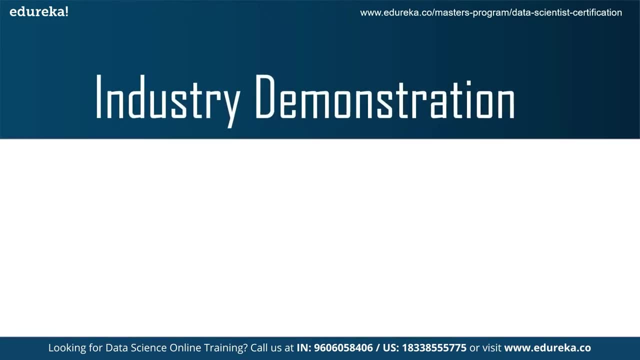 hypothesis testing is used in the industry and how the concepts which we have learned till now form an important foundation of useful industry concepts. So let's start. So till now we have done critical value method and p-value method, and both of them comes under z-test. 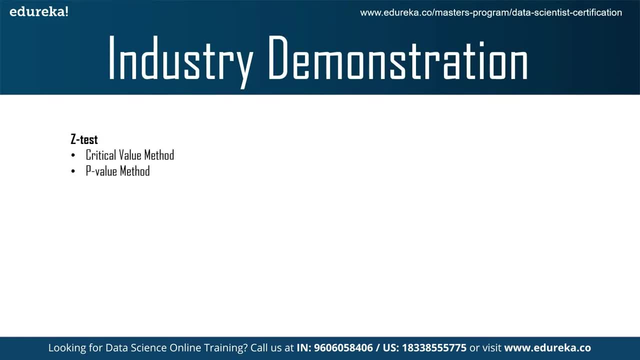 But what if I tell you that we won't be able to apply them practically, like when we are working in the industry? It happens because if you know the formula, if you remember the formula like it is, because the formula for standard error is population standard deviation sigma by square. 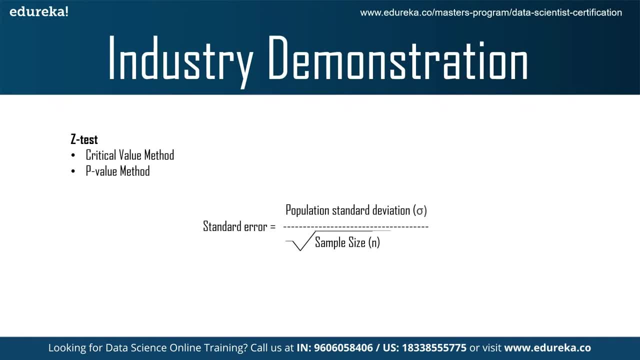 root of sample size n and in most of the cases, when we handling this the situation, practically we don't have the population standard deviation, so we won't be able to calculate the standard error. So how will we calculate the hypothesis? So here comes the t-test. 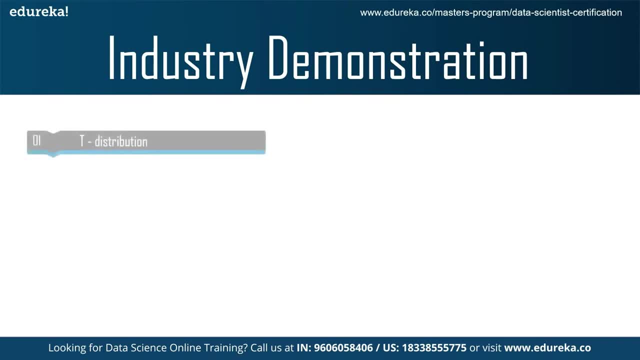 Before understanding t-test, first let's understand t-distribution. So if you see t-distribution, t-distribution's graph is actually very similar to normal distribution, Like you can see here: the normal distribution graph in blue and the t-distribution graph in. 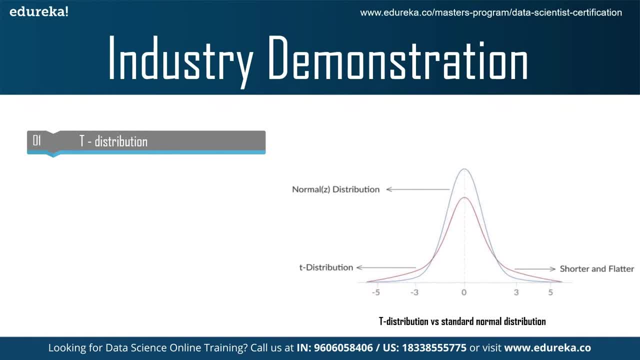 red. The only difference is t-distribution graph is shorter and a little flatter. So we can say: like t-distribution is a very similar to normal distribution. many cases, For example, like it is symmetrical about its a central tendency. However, it is a. 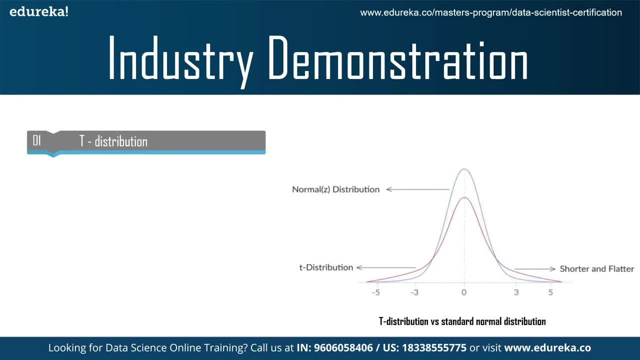 shorter than the normal distribution and has a flatter tail, which would eventually mean that it has a larger standard deviation and at a sample size beyond 30, the t distribution becomes approximately equal to the normal distribution. so each t distribution is distinguished by what statisticians call degree of freedom, which are related to the sample size of the data set. if 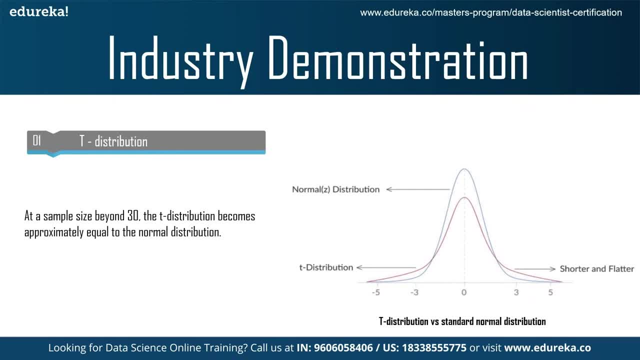 your sample size is n, the degrees of freedom for the corresponding t distribution is n plus 1. for example, if your sample size is 10, you use t distribution with 10 minus 1 or 9 degrees of freedom. you can say they note it as t 9, t base 9. okay, so smaller sample size, have flatter t. 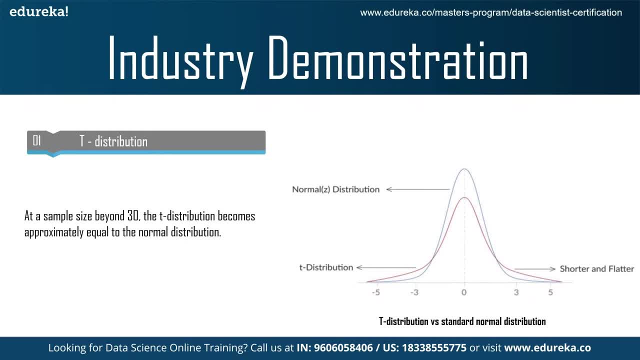 distributions than larger sample sizes and, as you may expect, the larger the sample sizes and the larger the degree of freedom. so, for example, if your sample size is 10, you use a t distribution with 10 minus 1, or say 9 degrees of freedom. so smaller sample sizes have flatter t distributions. 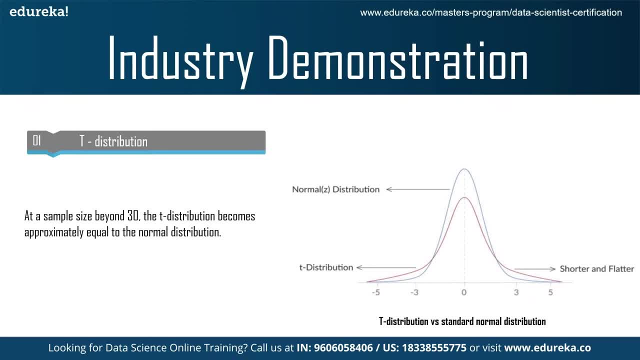 than larger sample sizes and, as you may expect, the larger the sample size is and the larger the degree of freedom, the more the t distribution looks like a standard, normal distribution. and the larger the degree of freedom, the more the t distribution looks like a normal distribution, or we can say the z distribution. so now the question is when t distribution is. 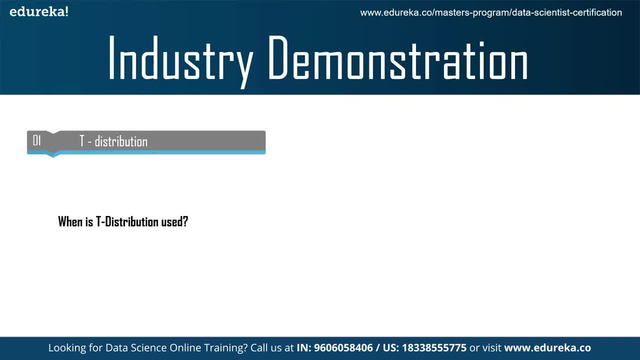 used. so the most important use of the t distribution is that you can approximate the value of the standard deviation of the population sigma from the sample standard deviation s. however, as the sample size increases more than 30, the t value tends to be equal to the z value. thus, if you 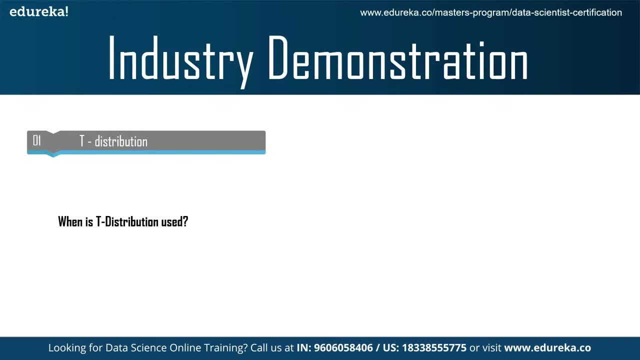 want to summarize the decision making in a flow chart. it will look like this: so if you look at how the method of making a decision changes if you are using the sample standard deviation instead of the populations, so if you recall the critical value method, the first step is like: calculate the value of zc from given value of alpha. that is significance. 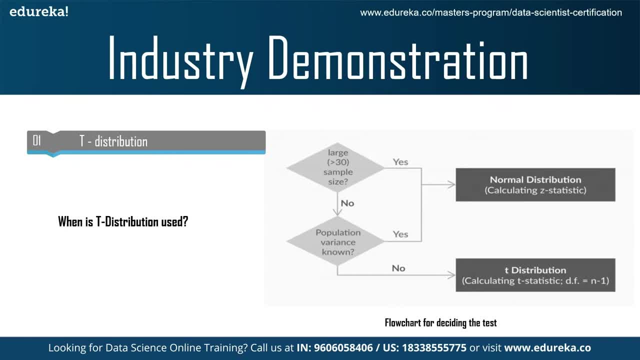 level. take it as five percent, if not specified in the problem. so to find zc you would use the t table instead of the z table. the t table contains values of zc from a degree of freedom and value of alpha, which is significance level. so zc in this case can also be called as t statistic. so practically. 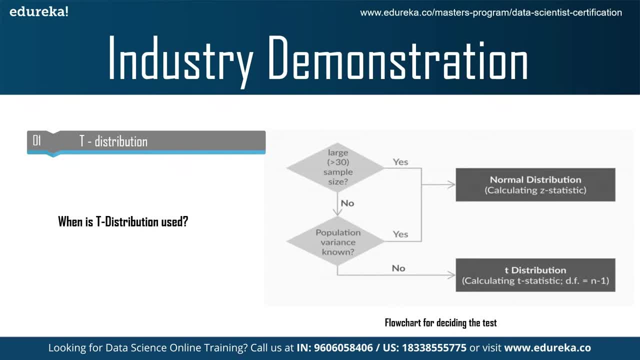 you would not need to refer to the z or the table when doing the calculation of the z table. so you need to refer to the z table when doing hypothesis testing in the industry. going forward, when you need to do hypothesis testing and demonstrations of excel or we can say of our programming, you 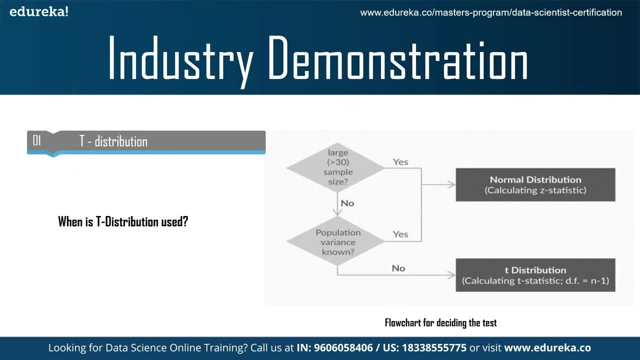 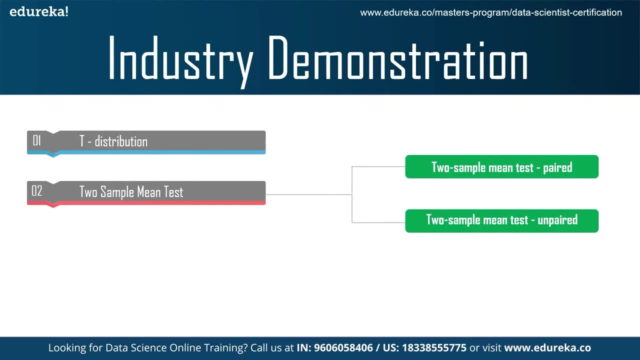 would use the term t test, since that is mostly performed in the industry. so all calculations and results of a t test are same as the z test whenever the sample size is greater than 30.. now the next one is two sample mean test. so two sample mean tests are divided into two types. that is a two. 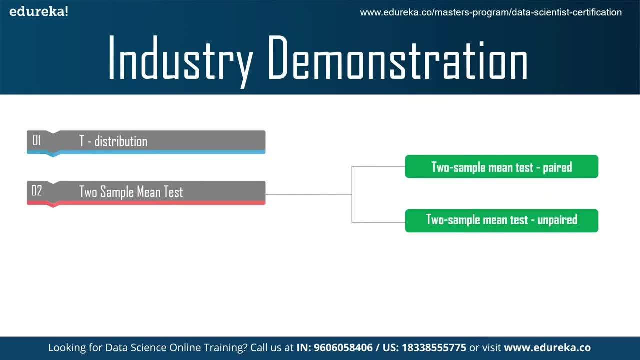 sample mean test and two sample mean test. unpaired test is used when your sample observations are from the same individual or object. during this test, you are testing the same subject twice. for example, if you are testing a new drug, you would need to compare the sample before and after the drug is taken to see if the results are. 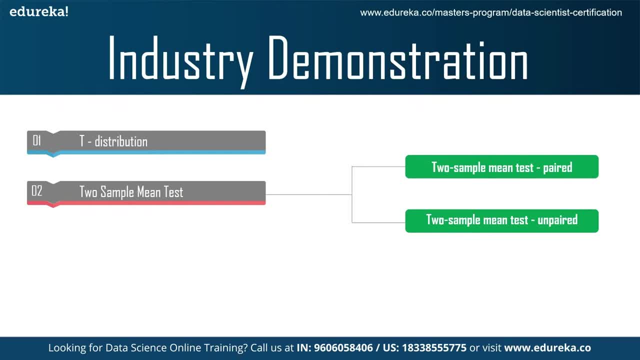 different and similarly for two sample mean test unpaired, which is used when your sample observations are independent. during this test. you are not testing the same subject twice. for example, if you are testing a new drug, you would compare its effectiveness to the that of the standard available drug, so you would take. 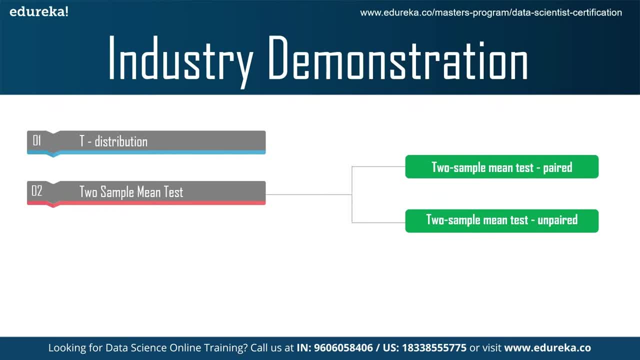 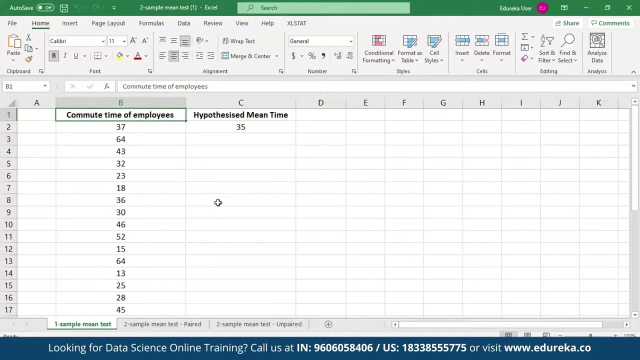 a sample of patients who consume the new drug and compare it to those who consume the standard drug. so we will do a test for it. we can do it in excel, so excel is like very heavily used in industry, so this is the data set we have. so we will be performing the t-test- multiple kind of t-test- in. 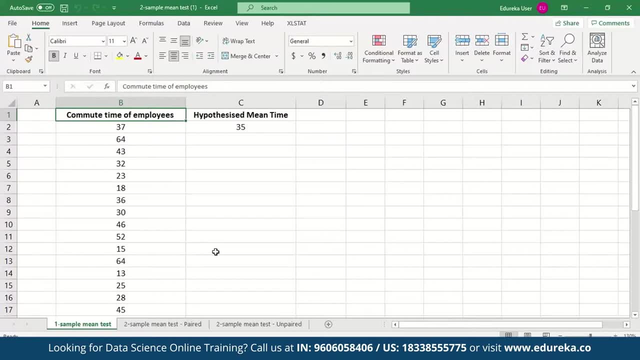 excel. so excel is like heavily used in industry for hypothesis testing. so first we can see the one sample mean test. in one sample mean test we have the commute time of edureka employees. we have taken the data of 32 edureka employees and we can see like how much time the employees 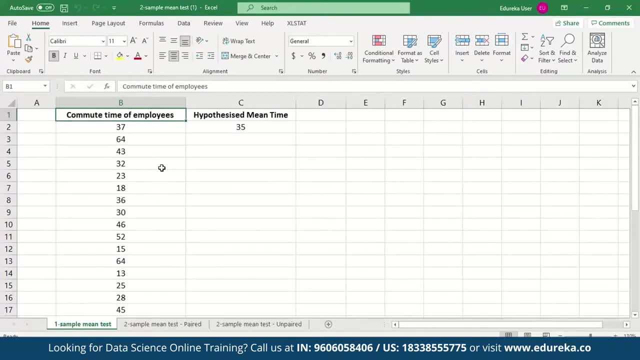 are taking for, like reaching edureka office from the respective homes and then reaching back to their home from the office. so we can say like this is the all the data for 82 employees and this is the hypothesis mean, which is 35. that means we can say the hypothesis, but we need to 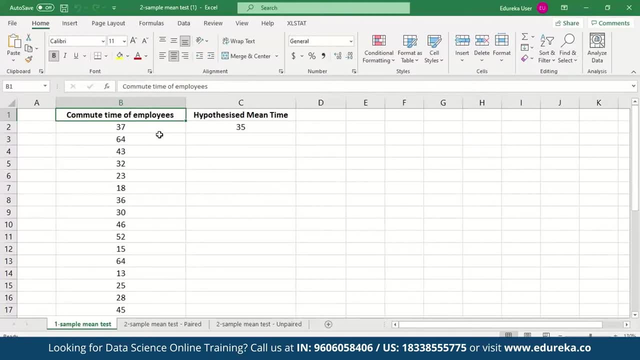 like do our research, along with the status we have to come the and prove the alternate hypothesis, whatever claim we want to make, like whether it is 35 or it is not. that is the sample we have previously seen in our like p-value approach and critical value method. also from our basic concepts which we have learned, we have learned how to do it. 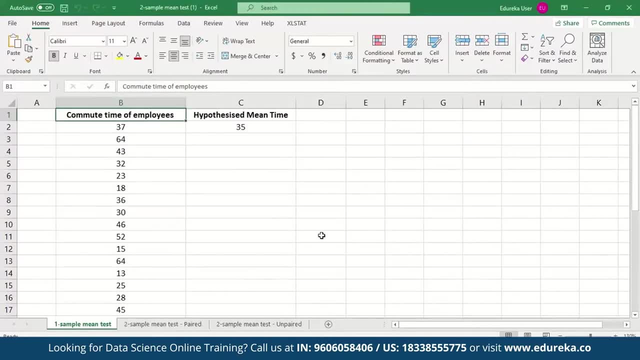 so this was the one sample mean test. now let's see the two sample mean test paired which we just talked about. so here you can see that there's a commute time for edureka employees, given for day one and also for day two for the same employees. that's why it is being called paired, because if 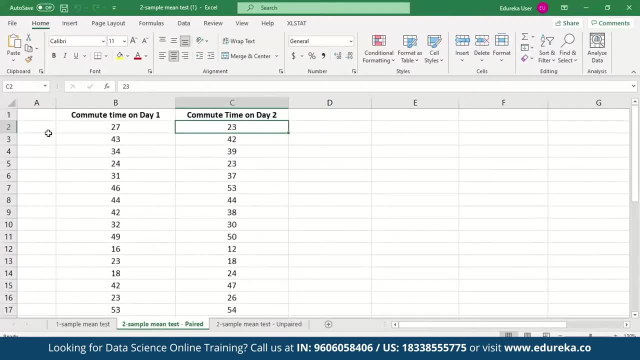 you see, the sample size is same and also of the same person. like. there's a person a, it has a on day one and a commute time of 23 on day two. similarly for person b, the same commit time of like 43 for day one and 42 for day two. so now what we have to do is we have to check for like whether 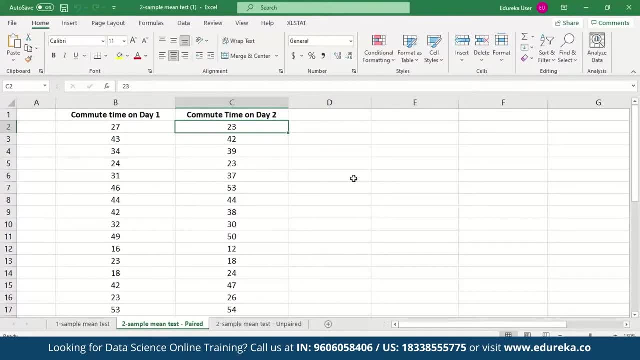 the average time is equivalent to: like, we have taken the average from your time to be 35. so if it is coming 35 or not for the day one and day two and we will find the difference. actually, the difference should be zero, actually, that then only the null hypothesis will be correct. so how we can. 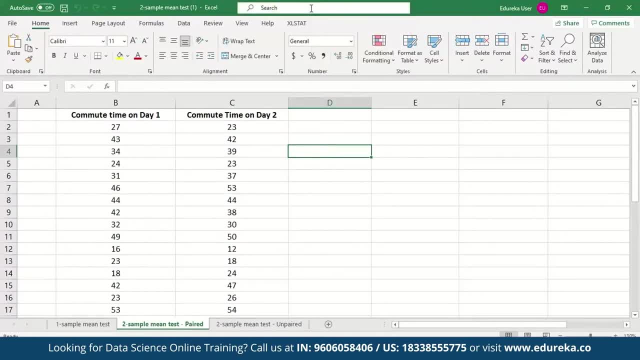 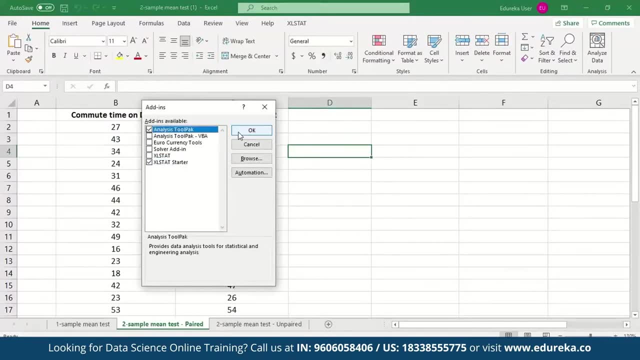 do is if you know like there is this option of add-in. so if you know like there is this option of add-ins, you can search for add-ins in excel. it is add-ins. you open the add-ins and you will find this option of analysis tool back. just select this one and click ok, and when you do that you will find. 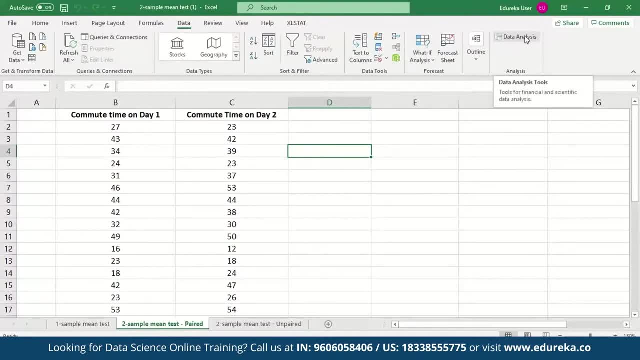 data option that there is a data analysis pack which has been added so you open this so you can see like different types of tests and different types of statistical methods are given here for checking. so here you can see like tms, t-test, paired two sample for means is given this one. 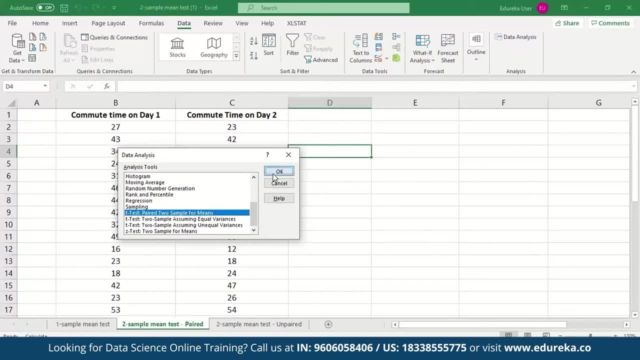 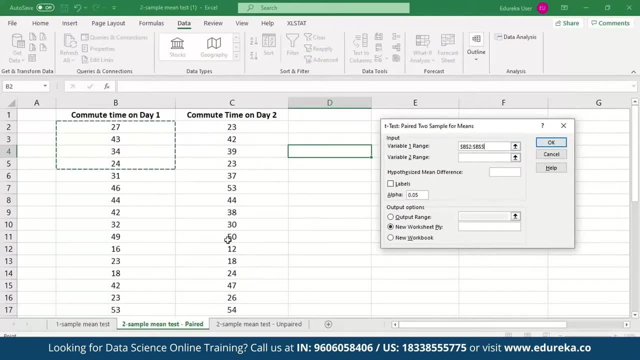 we have to select because we are checking for two sample mean test paired. so we'll go here and we will select the range. so let's see here, so range is from here down, this is the range and variable two, also range we will take. let's select here, okay, and hypothesize mean difference. 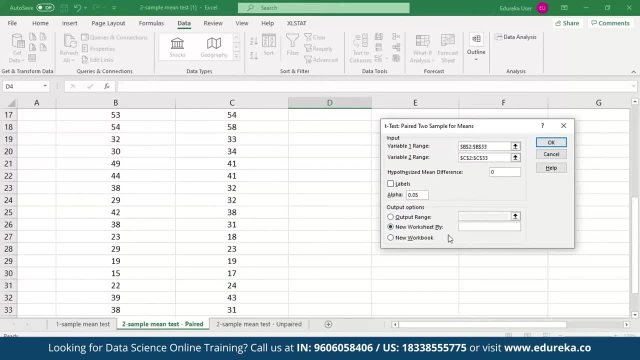 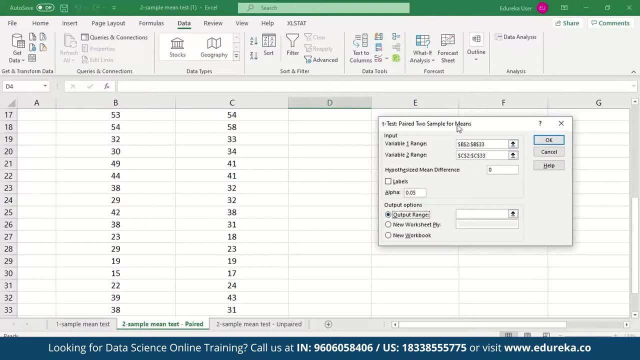 should be zero, right? so we will take zero and alpha value is 0.05. and output: you can also get the results in a new sheet, but other than that, you can also select the output range as well. in that way, you will get in the same sheet output range we can select. so 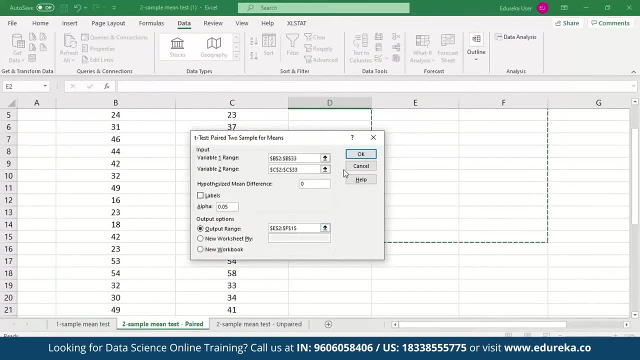 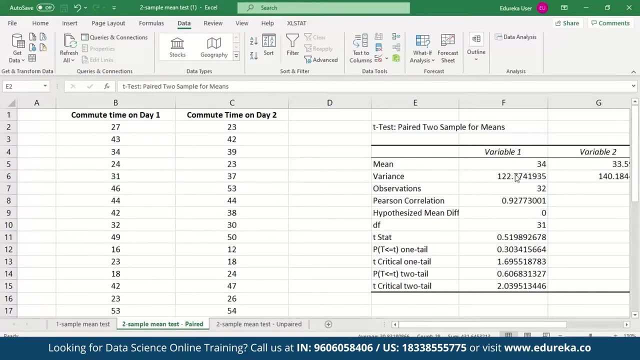 i will select column e and f, so that is the output range, and just click ok. so you got the results here. so you can see like that's just given a spare two sample for means and then mean. you can see like there's a little difference in mean for variable one and two and 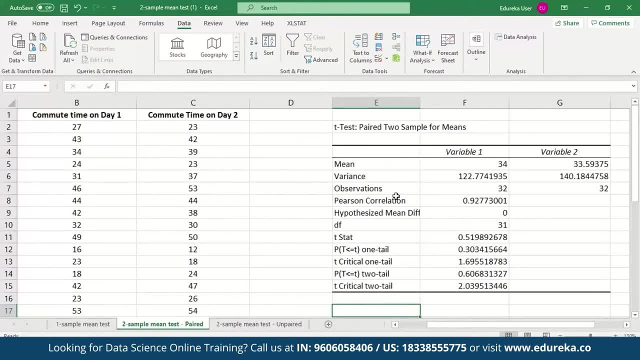 just a second. so other than that, the variance is also given. observations also, like you can cross track from here, like how many samples are given in variable one and variable two, so they are same, and pearson correlation is given and df is also given, t stat is given also like if it is a one. 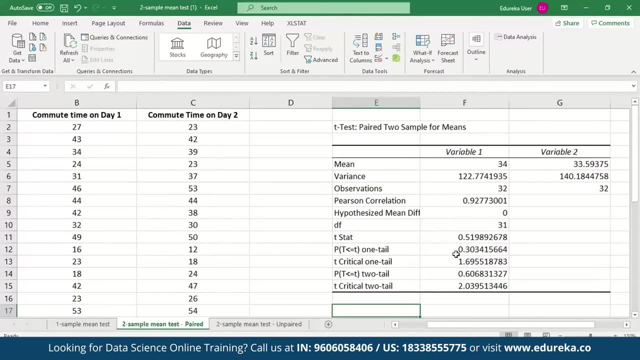 in that way, p value is also given. so you can see like even in one tail and two tail, both the values are larger than 0.05, and like 0.025 as well for two tail and one test in reference to that, and so we 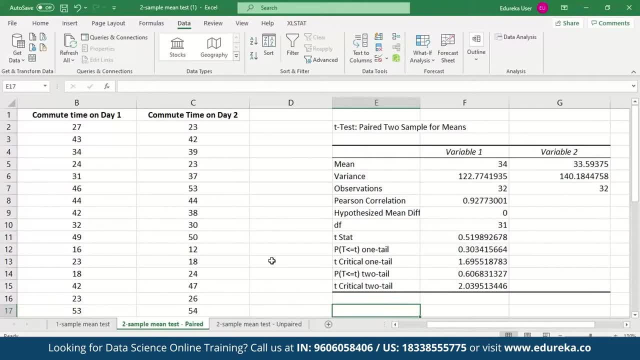 can easily say that if, comparing the value, the values of one tail and two tail tests are higher, so we fail to reject the null hypothesis and we don't have enough evidences to reject the null hypothesis. so that is the two sample mean test here. now let's come to two sample mean test, unpaired. 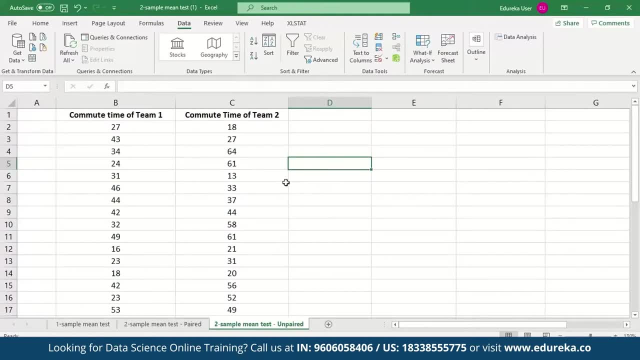 this one is. you can say like this is the commute time of for team. one we can say of, like this is for bangalore, for a direct of employees in bangalore and for edureka employees in new delhi, like in edureka employees in bangalore, the commute time is 27, 43, all these things are given, but it is. 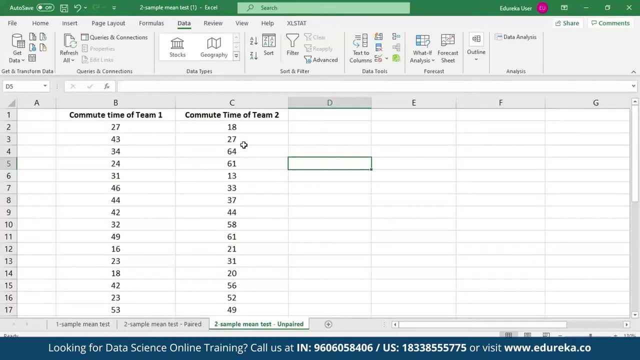 not related to team 2, which is in new delhi, so it's not of the same person. so that's why we say it as unpaired, because both the values are not related to each other. so in the same manner we can go and open the data analysis package. so there are like two things if you are sure about the equal. 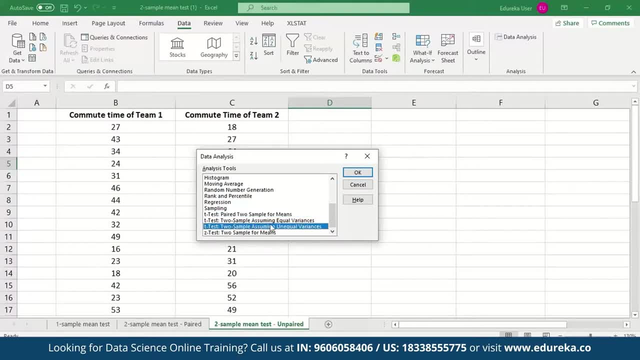 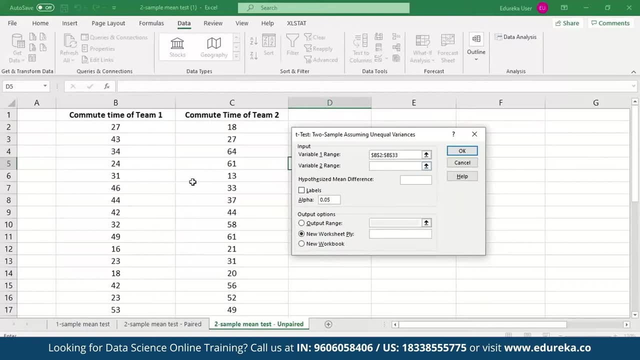 you can select, but right now i'm not sure, so i will select the t-test two sample, assuming unequal variance. so we will select this. we will select the variable range. and similarly, for second one, we are selecting this variable range per second. so for variable two, we will select the range. 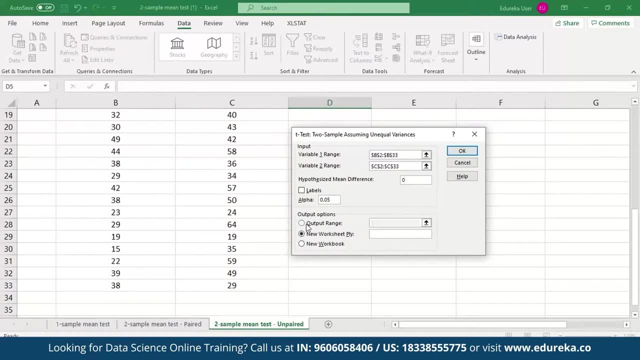 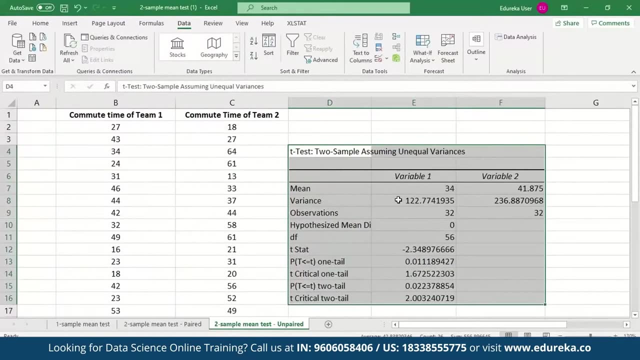 the difference will be zero here. we want in the output range, so we will select the output range as well. so let's select this. so that's it. so now you can see like the mean variance and everything, like there's a significant difference in me and you. 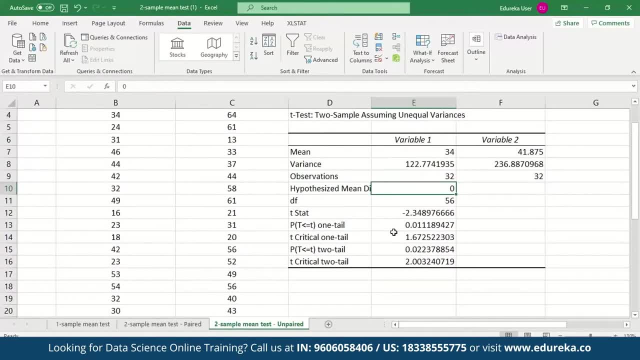 can see the variances there and everything, and for one tail test there's the value of 0.01, for two tails 0.02. so you can see like there is significant difference in that and it's also like lower the value of one tail test and two tail tests are lower than the 0.05 and 0.025 as well. so 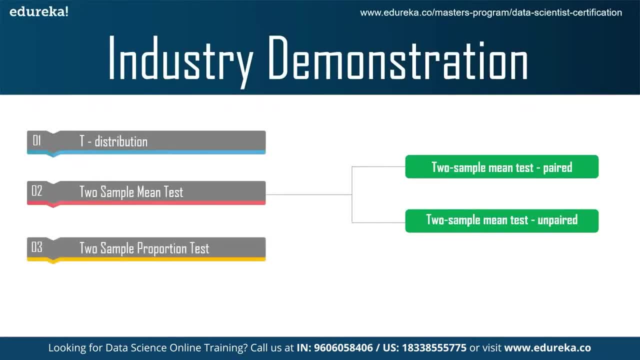 we can say like we are able to reject another hypothesis here. so now let's go back to the third t-test and that is two sample proportion test. so two sample proportion test is used when your sample observations are categorical, with two categories, like it could be true or false, one or zero, yes or 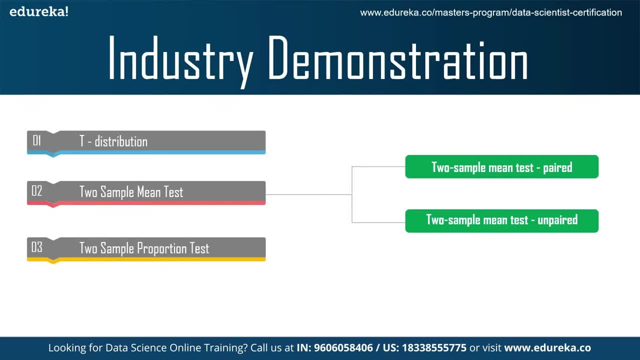 no male or female or we can say like success or failure, and they are like different other categorical examples. so, for example, if you are comparing the effectiveness of true drugs, you would define the desired outcome of the drug as the success. so you would take a sample of patients. 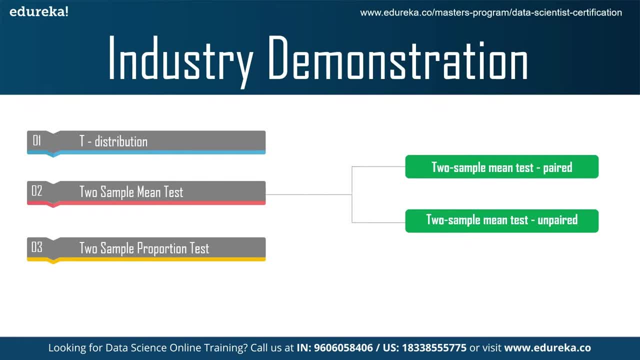 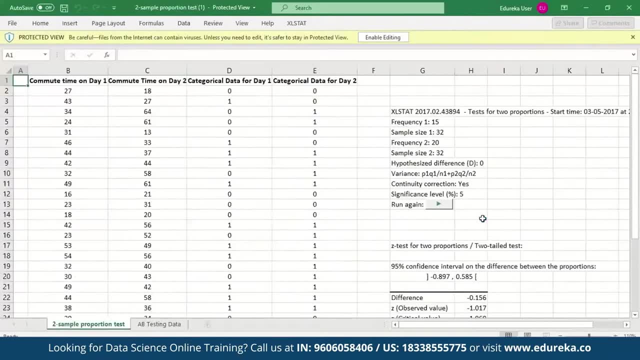 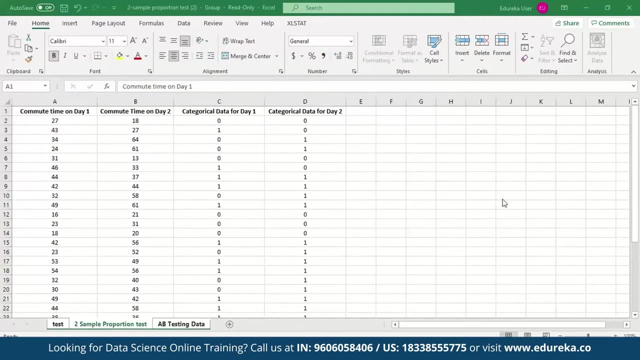 who consume the new drug and record the results of the drug and then you can see that, the results, the number of success, and compare it with successes in another sample who consumed the standard drug. so we will also see its demonstration in excel. so this is the data for two sample proportion test we are going to take. 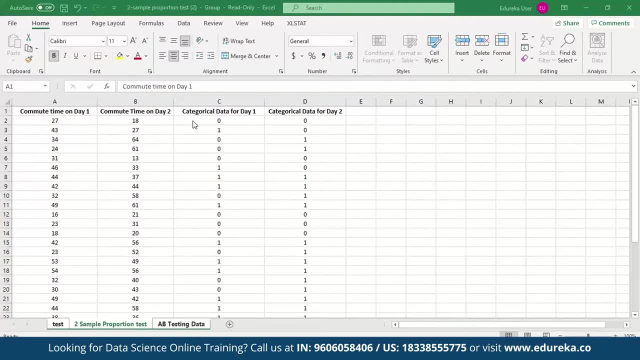 here you can say like: commute time for day one is given and commute time for day two is given, and then we have converted it and that into categorical data. so if the commute time is less than 35 it's zero, and if it is more than or equal to 35 it is one. so it's like the commute time is. 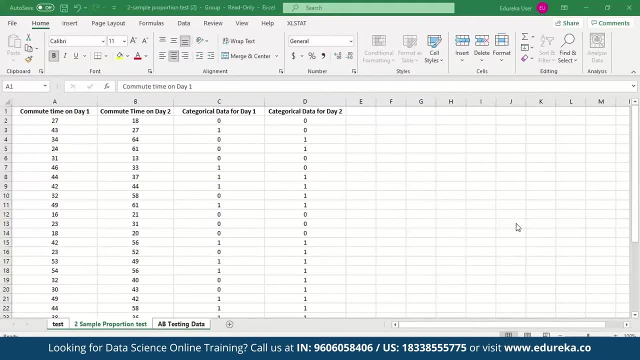 given in such a manner that if it is more than 35, it is one, and if it is less than or equal to 35, then it is zero. the data is given so here, but how we will gonna make the test, like execute the test here. this time we are not going to use the data analysis package. and there is one more thing. 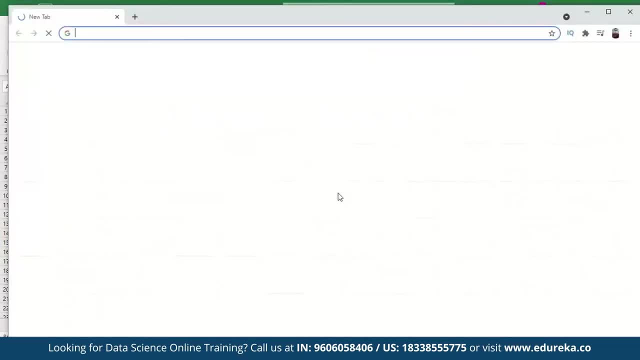 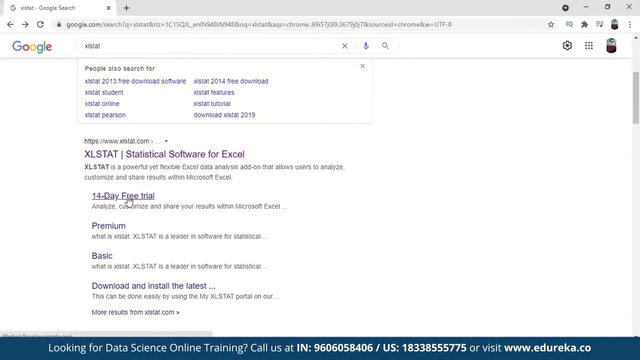 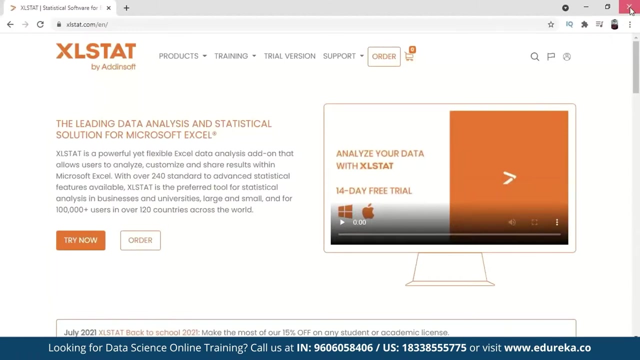 called excel state and for that you can like simply search for excel stat and you will get it for 30, so you can get a free trial of excel. start like it is a 14 tray free trial. you can click here and you can get it added to your excel. so i already have it added in my excel, so i will just go to. 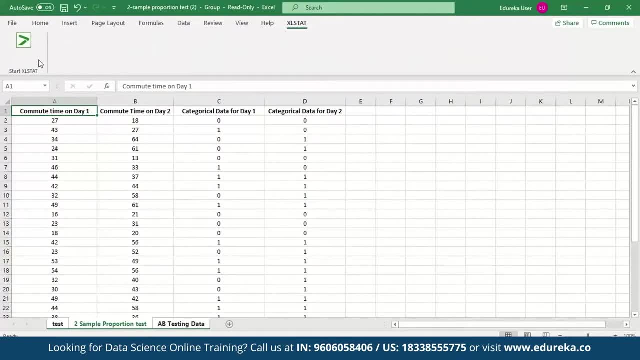 excel state here. here. this is the place where you where it get added. so you just have to start the excel stat first time when you click adjust your process and then again you have to go to excel state. then you can just go to test a hypothesis and that you have to go to parametric tests and 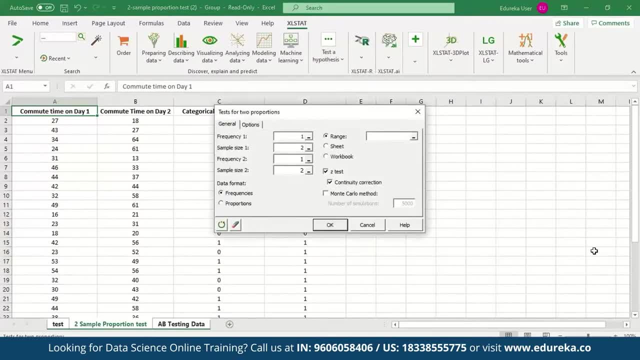 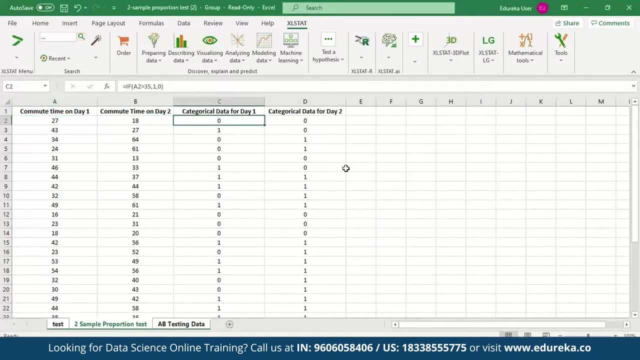 select the test for two proportions, so you have to select the frequency for it. just a second, we will just cross it. we will first select the frequency, we will first take the frequency for it. so same data power. so here you can see: the frequency is 15 and the total sample size is 32, and in this one frequency is 20 and the 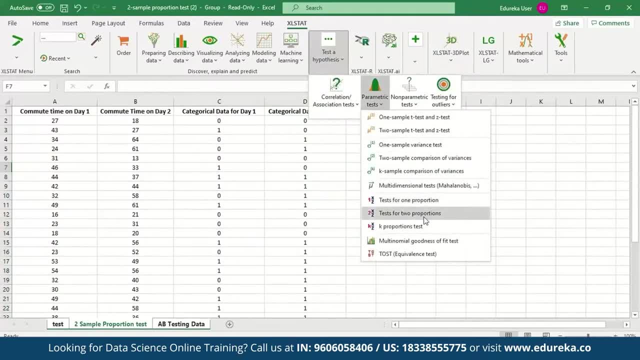 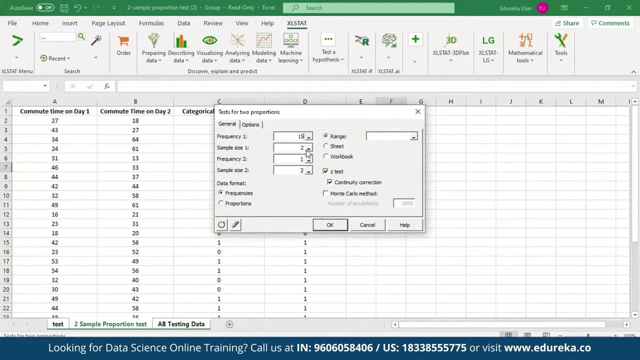 total sample size is 32.. so we'll again go to parametric test two proportions and we can now give the frequency right. so it is just 15 and this is 32 sample size. this is 20. sample size is 32.. we can also select the proportion as well, but we will be like: 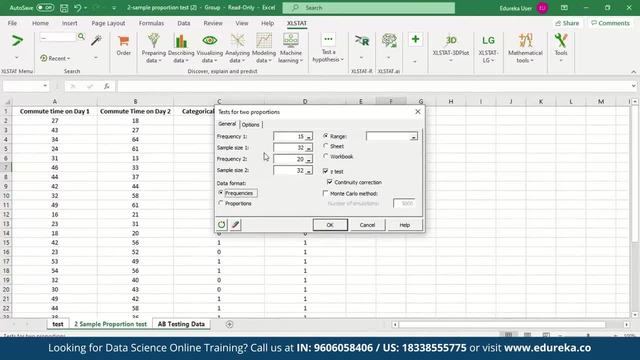 selecting the frequencies only, not proportions. so, because it's easier, so, and again, we can like select the range for it. so we will just select the range and you can select. in this manner, the range has been selected. other than that, you can go to the options and here the hyper size reference will. 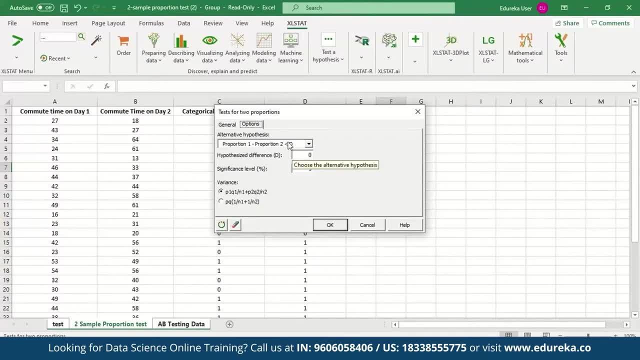 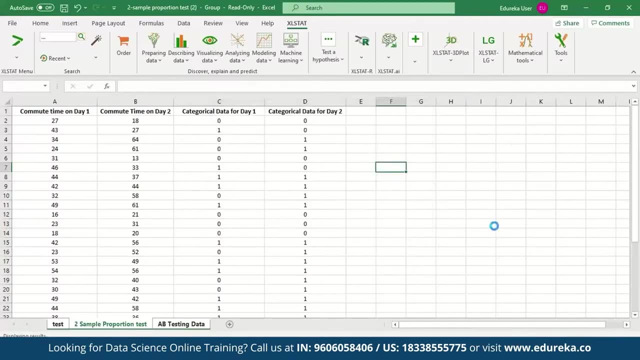 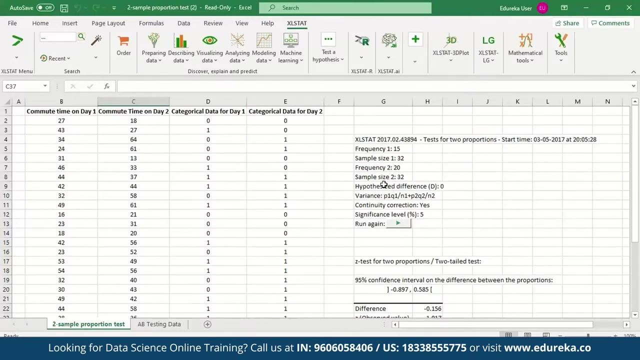 be zero, significance will be there and variance will be there and in this we have to like, select the like proportion where minus proportion two is uh not equals to p. that is the one hypothesis. so we will just select. okay, so now you can see like we got the results. so you can see like the frequency is going to 15 samples- i was 32. 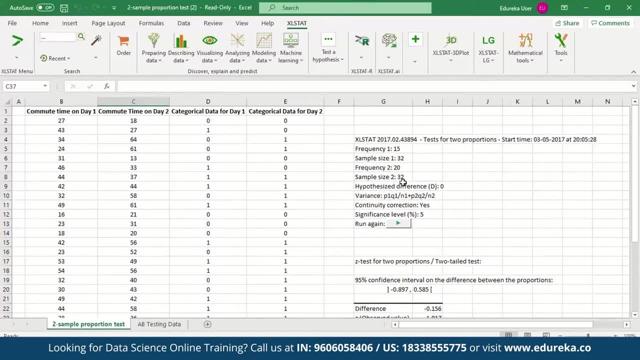 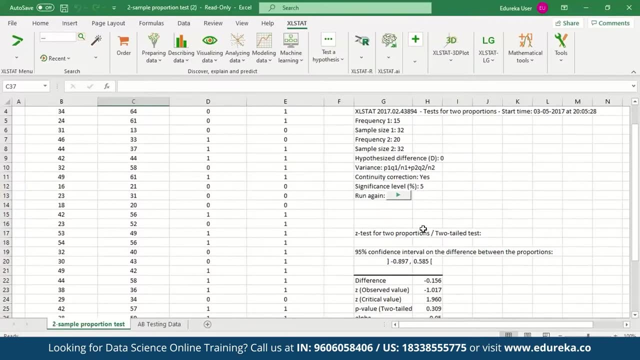 frequency. everything is given sample size 2 in the same frequency and the same sample size, same minute is given. also like, if you want to run again with a different frequency, that also you can run, that's not a problem. so if you like want to change, the alpha value means the significance. 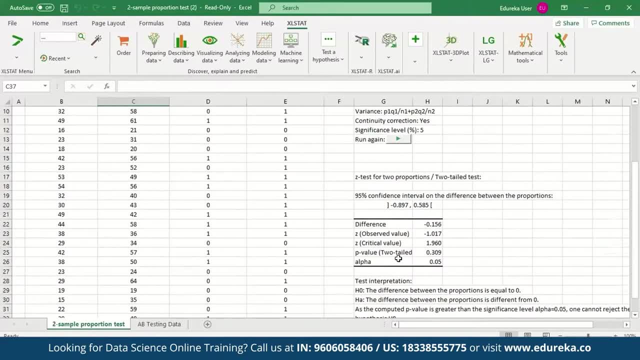 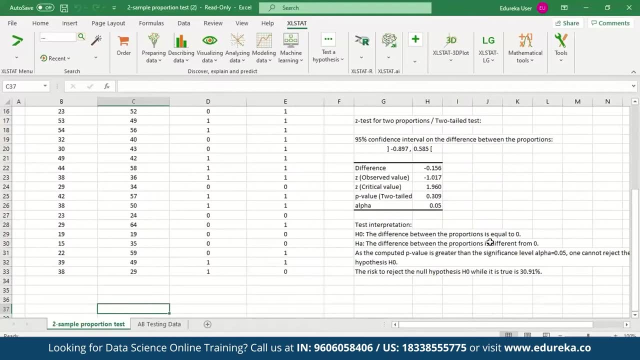 level. you can change that and again run and you can see the difference is given. so we see that the difference between the proportion is equal to zero and the difference between the proportion is different from zero. that is the alternate hypothesis. but as the compared p value is, 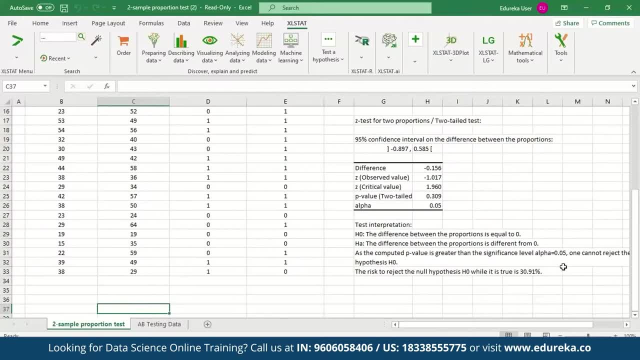 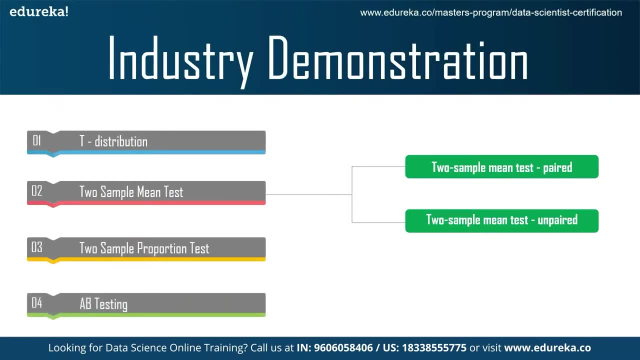 greater than the significance level. so we cannot reject the hypothesis. so we got the answer here, so now let's move on to the next test. the next test is a b testing. so a b testing is like a direct industry application of the two sample proportion test sample while developing an. 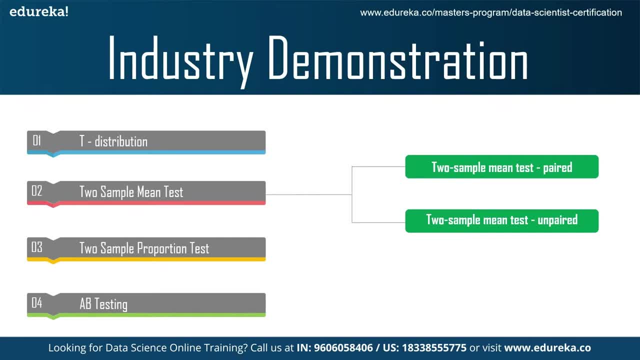 e-commerce website. there could be, like, different opinions about the choices of various elements, such as the shape of buttons, the text on the call to action buttons, or like the colors of various ui elements, or, we can say, like the copy on the website or numerous other such things. so often, the choice of these elements is very subjective and is difficult to predict. 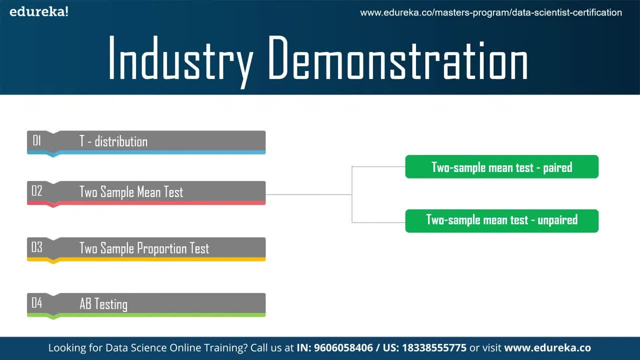 which option would perform better. so to resolve such conflicts, you can use a b testing. so a b testing provides a way for you to test two different versions of the same elements and see which one performs better. so every testing is like: entirely based on the two sample portion test. 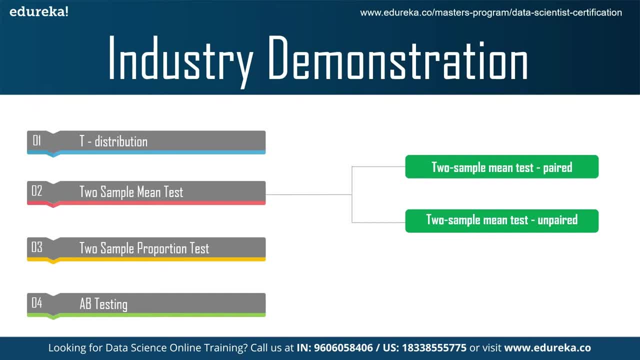 is used when you want to compare the proportions of two different samples. you can use various tools to conduct kb testing, like r or optimizely, etc. so but here we will be doing the same: a- b testing in excel. you can like use various tools to conduct a- b testing, like optimizely, excel, etc. 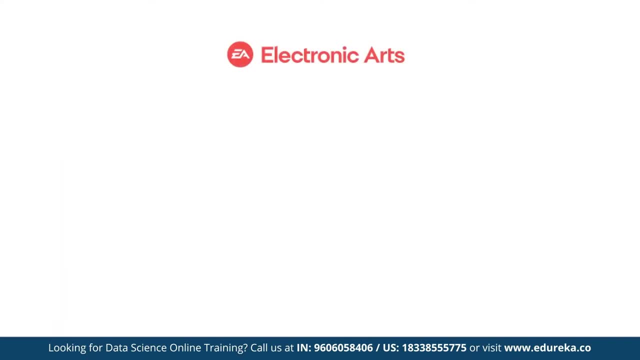 so let's see an example of a- b testing, like: if you know, like there is this media company like gaming company electronic arts. so when electronic arts, or successful media company, released a new version of one of its most popular games, like ebay, gaming company, electronic arts is a media company. 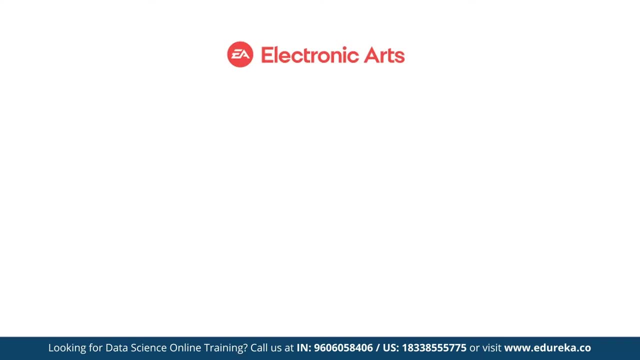 the company wanted to get it right, which is the simcity 5 game. so if you see the home page for simcity 5, a simulation game that allows players to construct and run their own cities would undoubtedly do well in terms of sales. so electronic arts wanted to capitalize on its popularity, so 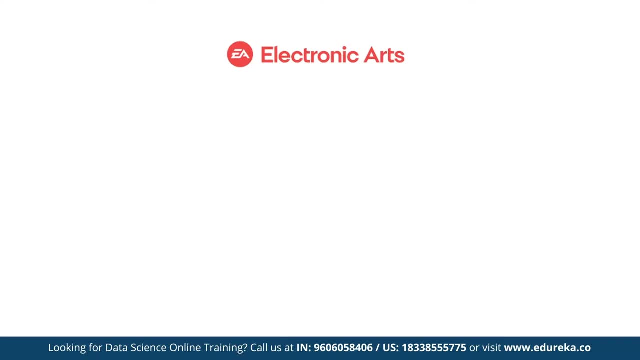 according to like hubspot, electronic arts relied on av testing to get its slide page for simcity 5. just right. so the desire behind this av testing example revolved around improving sales. so electronic arts wanted to maximize revenue from the game immediately upon its release, as well as 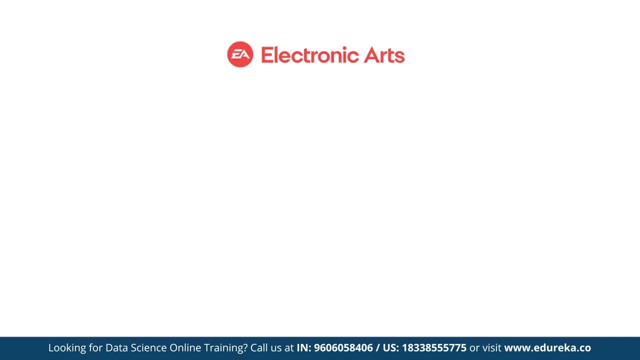 through pre-sales efforts. so these days people can like buy and download games immediately. the digital revolution has made those plastic encased cds nearly like obsolete, especially since companies like electronic arts promoted digital downloads. it's less expensive for the company as well and like more convenient for the consumer. so, however, sometimes the smallest things can like influence. 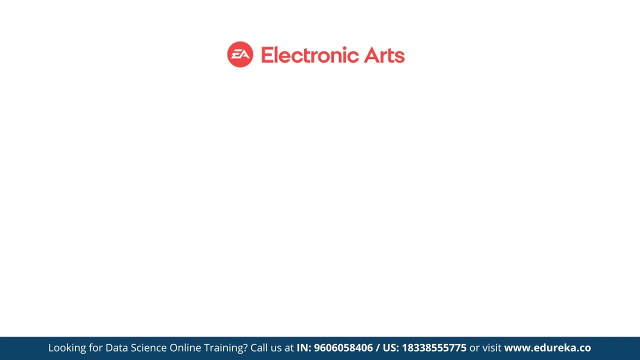 conversions. like electronic arts wanted to test different versions of its sales page to identify how it could increase sales exponentially. so i'm highlighting this particular a b testing example of simcity 5 because it shows how hypothesis and conventional wisdom can blow up in your faces. so, for instances, most marketers assume that advertising incentive will result in increased. 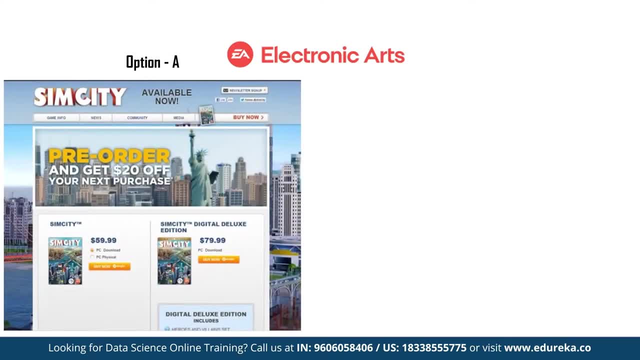 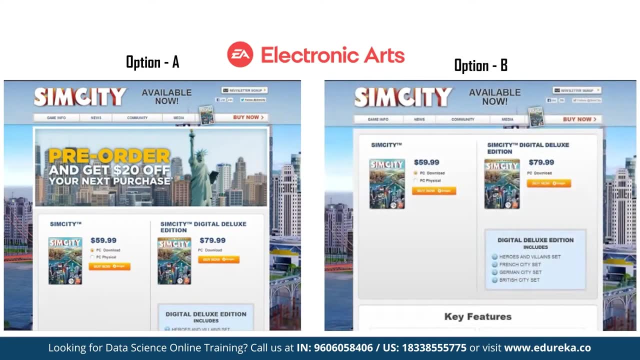 sales. that's often the case, but not this time. so the original version of the pre-order page, which you can see here, has offered 20 off on a future purchase for anyone who bought simcity 5, and you can see the option b. so which is the variation, which is a like created afterwards? 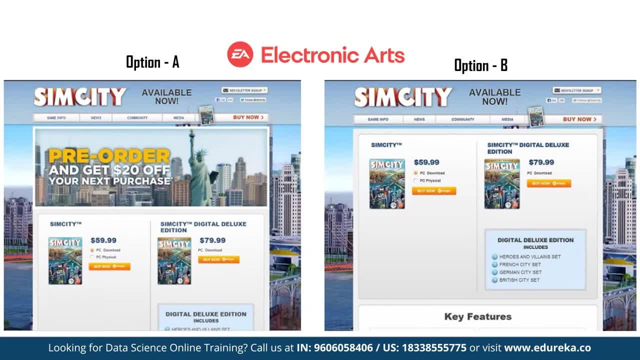 the variation, if you see like, has eliminated the pre-order incentive. here the pre-order incentive is given and here there's no pre-order incentive. so, as it turns out like the variations performed more than actually, 40 better means option b performed 40 better than the control version means the original version. so avid fans of simcity, 5. 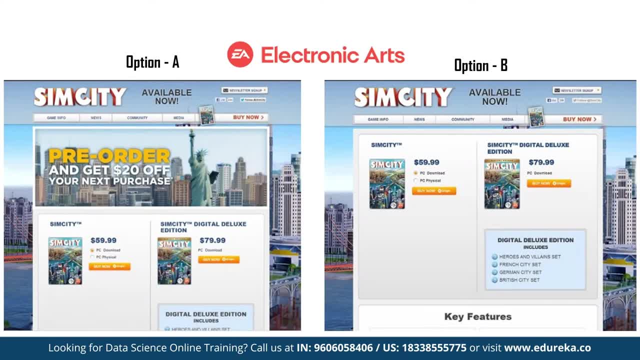 weren't interested in an incentive, so they just wanted to buy the game. as a result of the a b test, half of the game sales were digital, so do you understand why it works? so the a b test for electronic arts revealed important information about the games audiences. like many people who 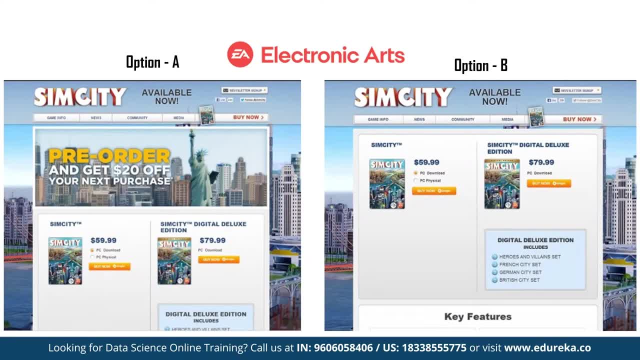 like simcity don't play any other games. they like this particular franchise. consequently, the 20 of offer didn't resonate with them. if you make assumptions about your target audience, you will eventually get it wrong. so human behavior is like difficult to understand, even without hard data. 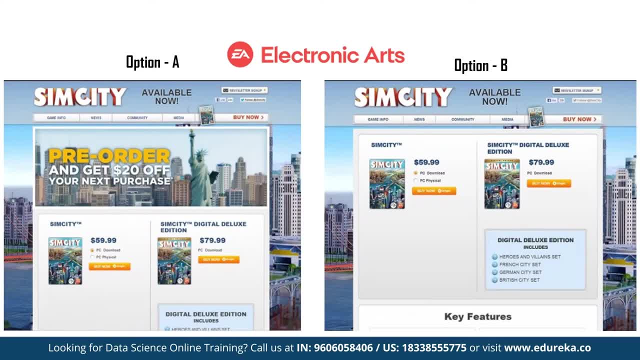 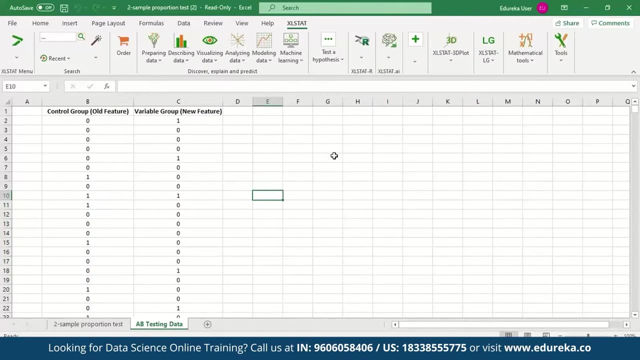 so you need a b testing to generate data on which you can rely. so let's now demonstrate a b testing, also on the same excel file. we have the data set already, so we will just go to a b testing data. so you can see the data is given here for control group and variable group. so we can say like this: 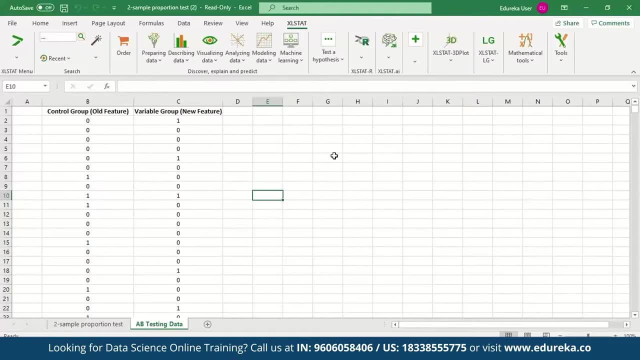 is for our adreca website only, for example. so like someone has reached our website and has opened the course, and if that person registers on the application, so that is where we give them as a one, and who haven't registered, we give them a zero. that is how it has been labeled, that's how we have. 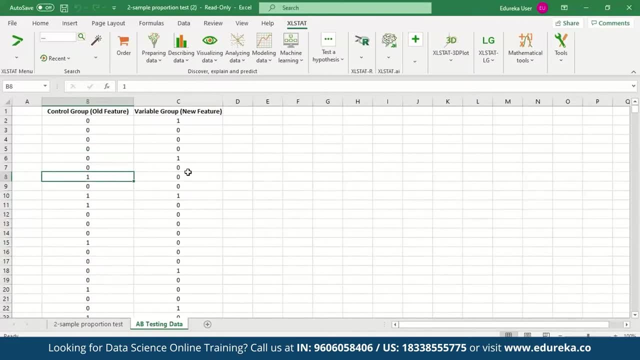 labeled the data. whoever has registered, it's one, and whoever has not registered and but has opened the course, we have labeled it as zero. let's not check it out, let's just go ahead and check it out, the results for both of them. so let's go to excel, start and same visualizing data we can open, not 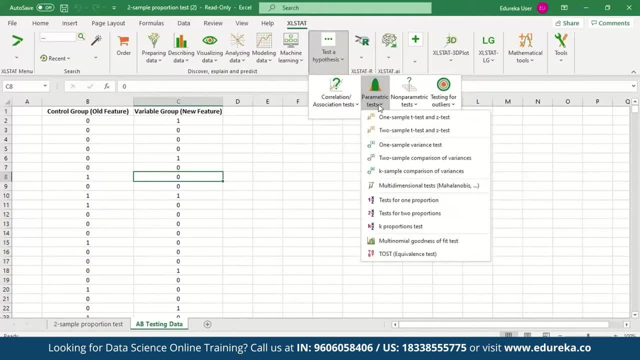 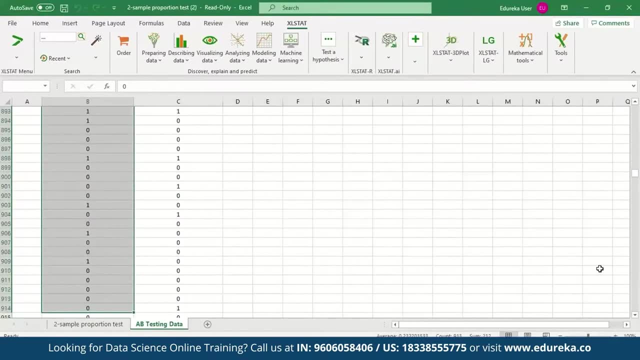 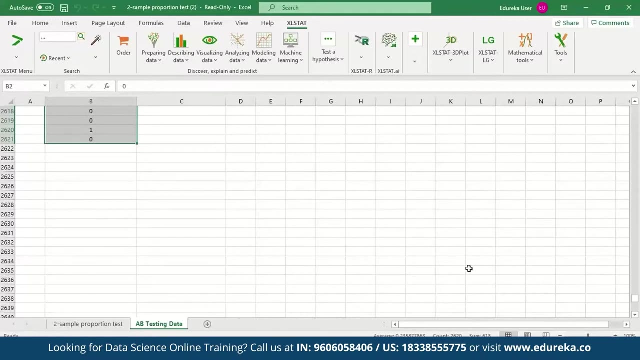 the visualizing. so test our hypothesis and we can go to parametric tests and we can do the same test for two proportions. so first let's check the frequency of it, so you can see: the total sample size is 2620 and sum is 618. so we will just select it here, we will just copy it here: 618 and 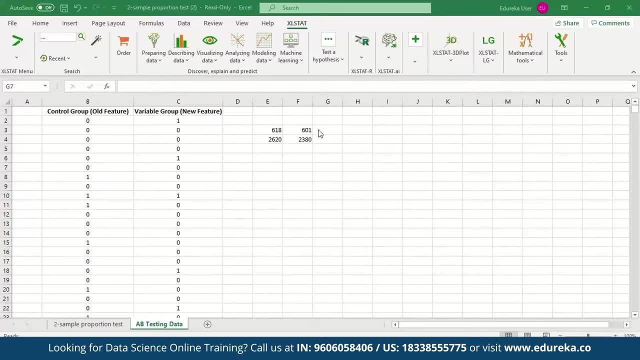 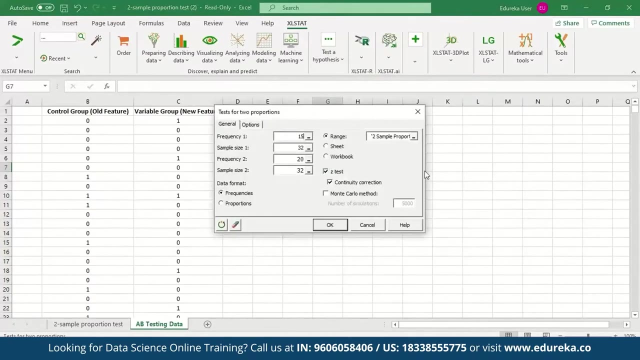 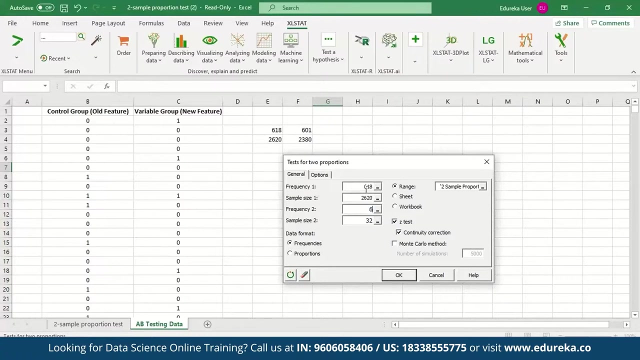 620. so similarly we will do the count for variable 2 also and we got like 601 and the frequency and the 2380 as a sample size. so we will just go to test a hypothesis, to parametric test, test for two proportions. we will just fill the values here: 618 and this is 2620, this is 601, this is 2380. 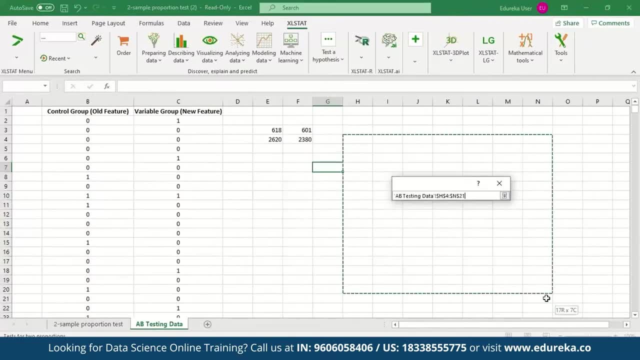 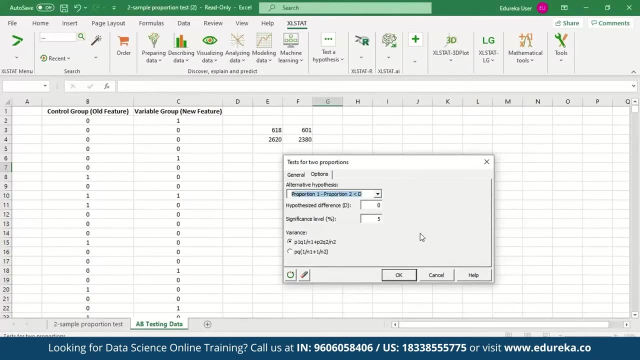 select the frequency and then we will select the range as well. like this range and other than that, we will go to options, and for this one we will select the proportion minus. the proportion 2 is smaller than d which is lesser than 35. that is our null. 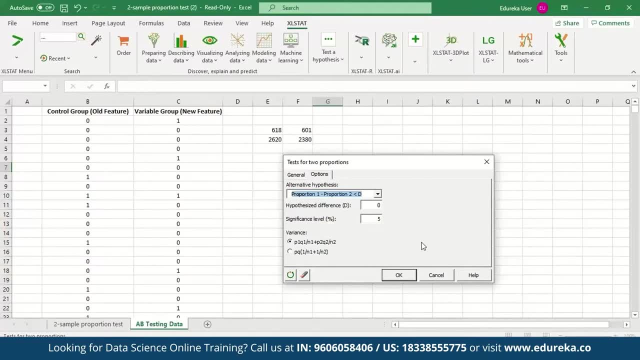 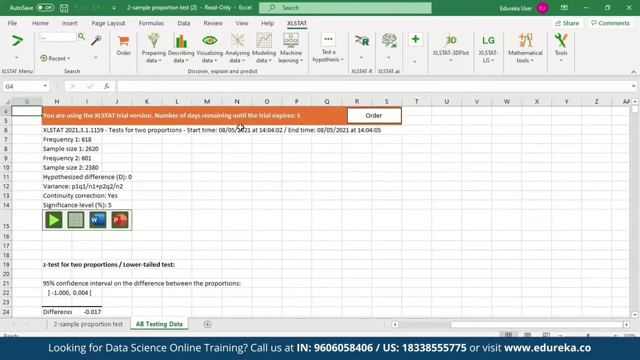 hypothesis and everything is same like 0 and significance, table 5, and then we will just give okay, so results will be here soon. so yeah, as i am using the excel start trial version, so it is showing like to use the trial version. so yeah, so you can see, here is like test for two proportions. 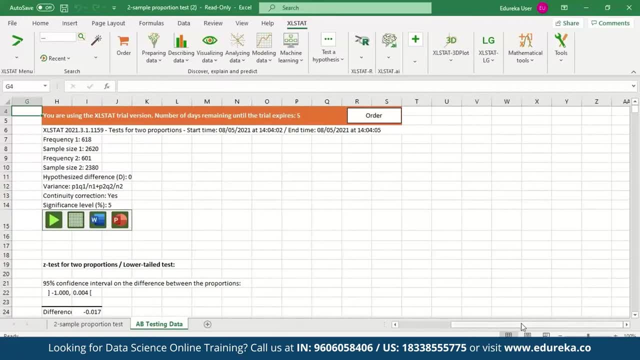 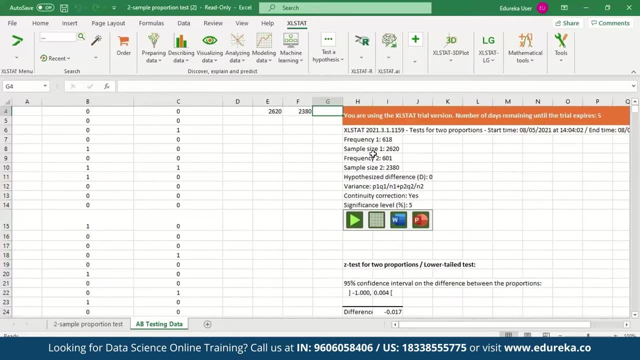 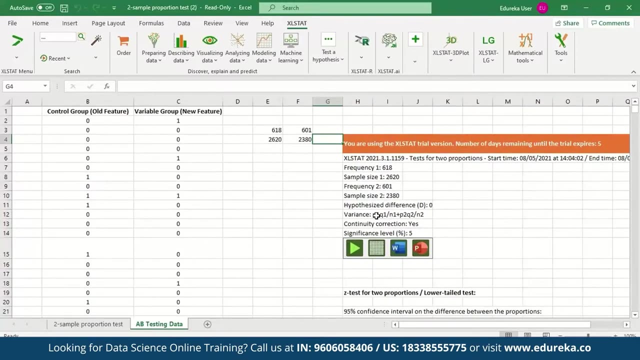 we have done, which is the av test. but you can see like the frequency and everything is given here. frequencies, you can see like 601 out of 2380 and so if you calculate it in percentage, for the variable one, that is for control group, there is a 23 success and for the sample size, 2, which is 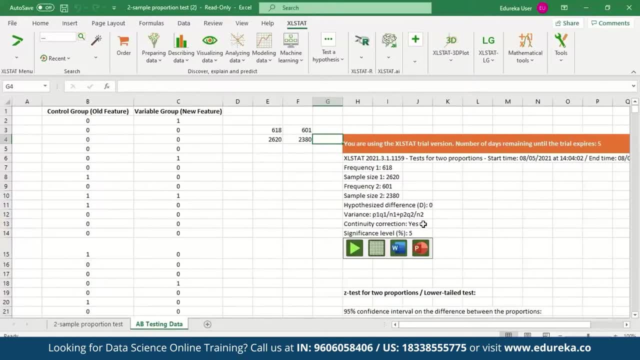 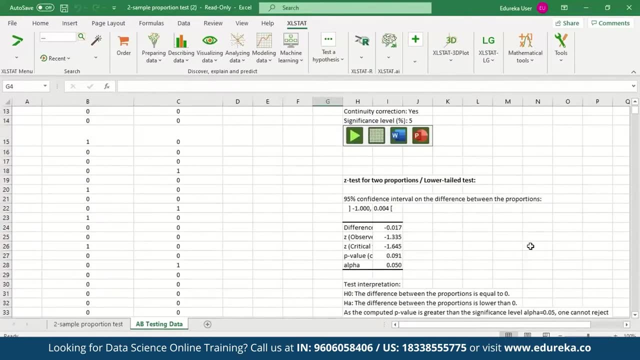 like variable group. for that the success rate is 25. so we found the variance also like continuity correction, everything is the data is given and like 95 confidence interval on the difference between the opportunities we have got and you can see like the p values, 0.091, which is like the an. 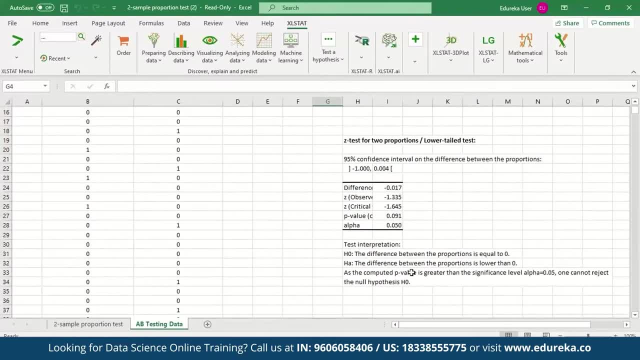 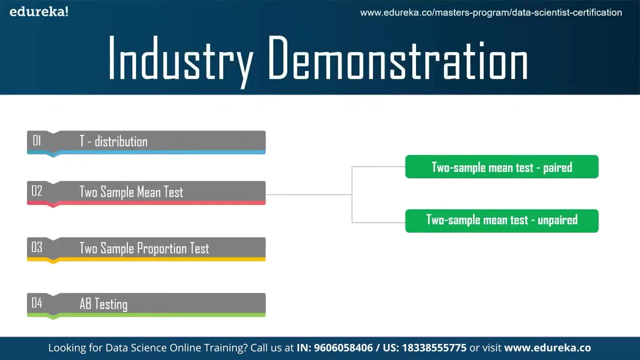 0.05. so we see like p value is greater than alpha value. so the answer is like we cannot like reject the null hypothesis because like p value is greater. so that's how the a b testing is done. so now we are like done with all the testings and we have completed the industry demonstration as